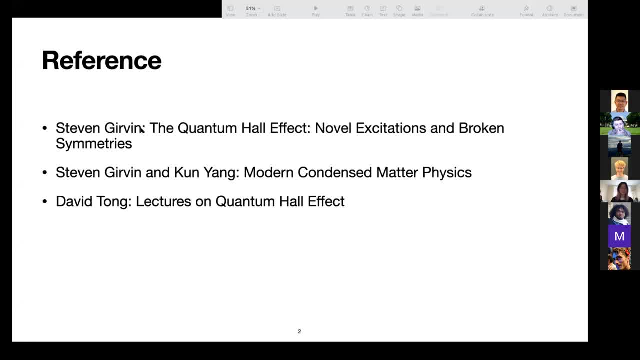 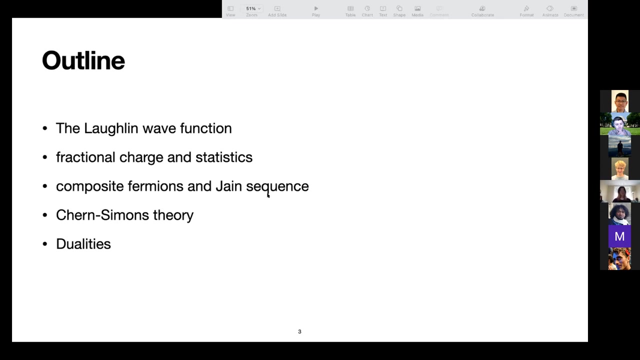 such as the lecture notes by Stephen Gervin and the chapters in this book by Gervin and Young. There are also lecture notes by David Tong which are very good. So today I'll be- this is my outline- So I'll be talking about some basic stuff of fractional quantum Hall and an effective field theory, which is a transcendence theory. 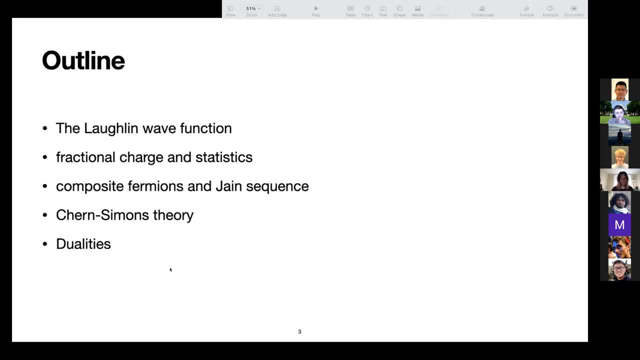 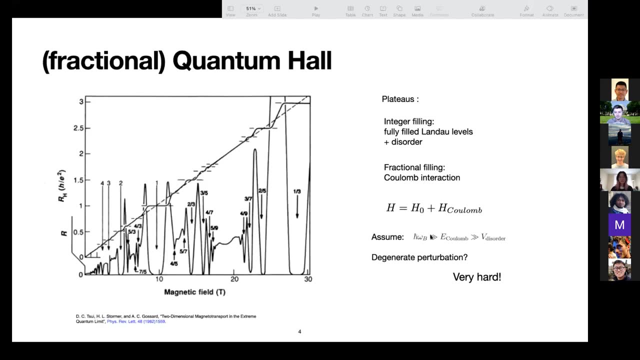 And if I have time, I'll talk about dualities and to make contact with previous journal club topic by Robert. So let's get started. So this is the famous Hall measurement. So, as we can see, there are some plateaus in Hall conductance at integer fillings, which are called integer quantum Hall effect. 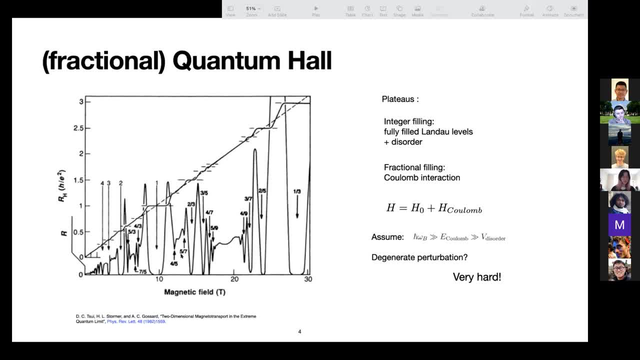 And also as some fractional fillings. So we are all familiar with integer quantum Hall. Basically it can be explained by fully filled Landau levels of 2d electrons, 2d electron gas and magnetic field and plus some disorder which caused the plateau. 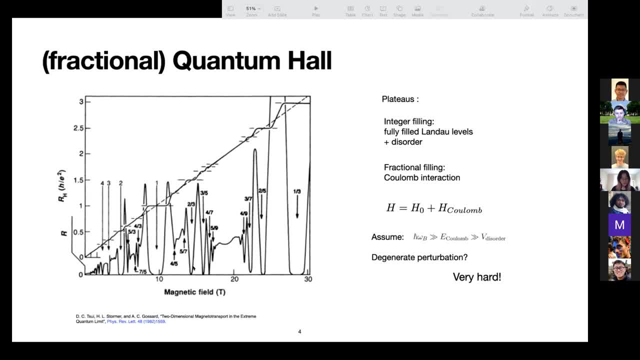 But so for fractional filling. it's a little bit weird, Because if we consider, consider a partially filled Landau level, since there's no, I mean if we do not include any electron-electron interaction, there's no way we can get an incompressible state. 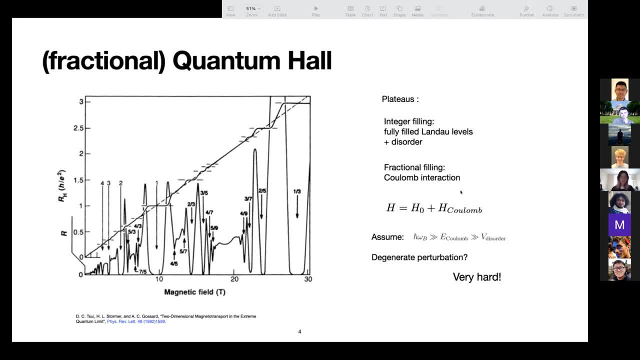 So that means Coulomb interaction must be very crucial in this fractional quantum Hall context. So during the, so for the rest of my talk I'll assume this hierarchy of energy scales, which is disorder, much less than the Coulomb interaction, much less than the Landau level splitting. 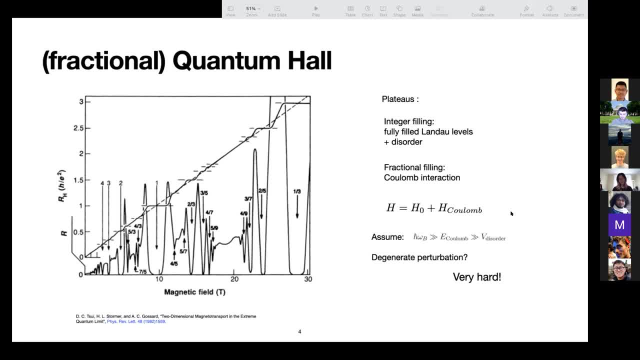 That will allow us to work with the projected states living in, say, lowest Landau level or a few Landau levels and ignore the Landau level mixings. So with that, the Hamiltonian we're considering is basically basically contains two terms. 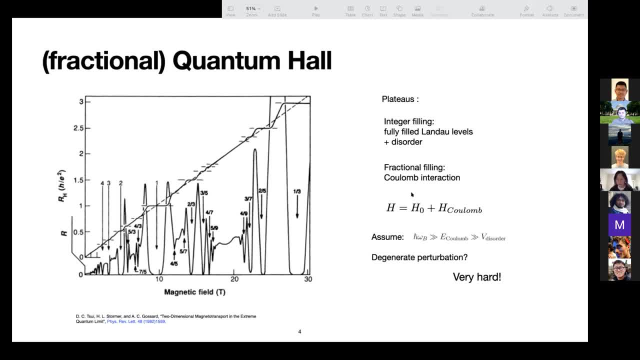 One is: well, it's some electron gas coupled to the Coulomb interaction And the electron gas coupled to an external magnetic field. We all know how to solve that. It will give us Landau levels. The other one is a Coulomb interaction. 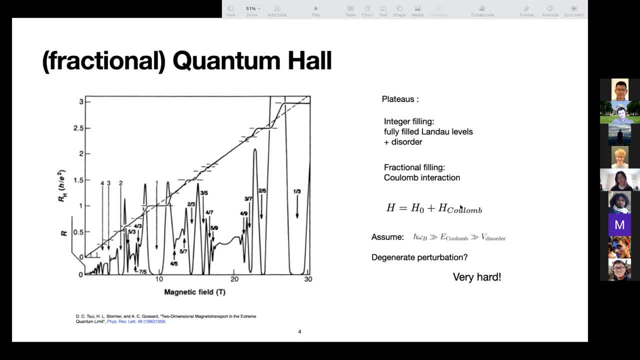 So we are taught to do perturbation theory during our like in the grad courses. But notice that if we have a fractional filling the ground state degeneracy of this, the ground state of H naught, their degeneracy is huge. 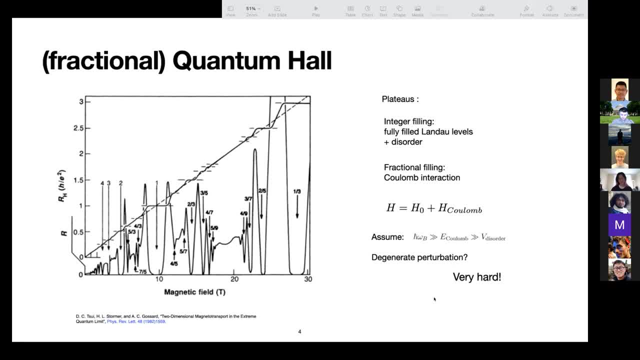 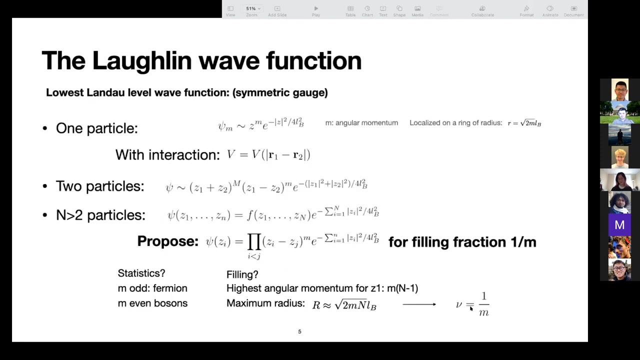 So it's a very hard problem to do a degenerate perturbation. But so so Laughlin made a very bold move. He's like: how about I just guess the ground state wave function directly? I mean, after all, that's what we want. 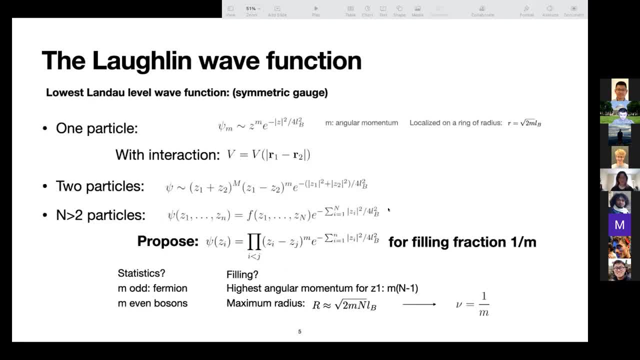 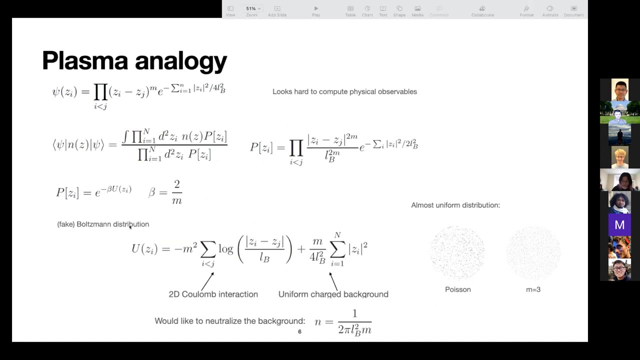 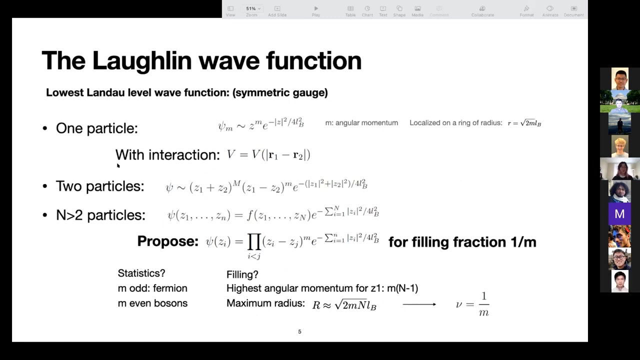 So, yeah, so, so let me introduce the gas wave function, which is the Laughlin wave function, And, yeah, let me just motivate how? let me just motivate this, sorry. Yeah, let me just give you some motivation. So for, if you, if we consider a single particle state, 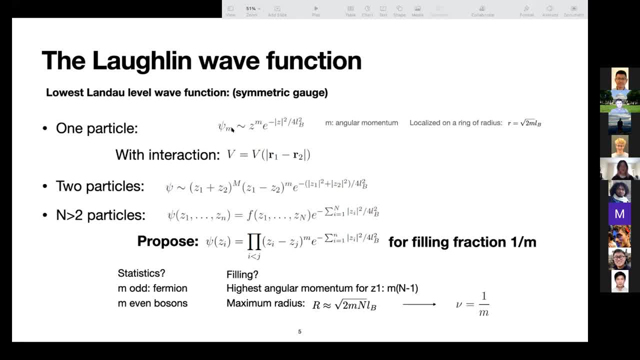 the wave and assume, assuming symmetric gauge wave, the wave function for lowest Landau level is just some holomorphic function times, an exponential decay component. So the the power here m is actually actually labels angular momentum And this wave function actually localized on the ring of radius. 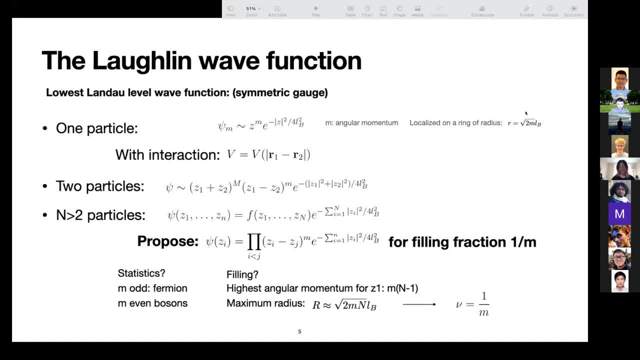 which is square root of, proportional to the square root of m and times the magnetic lens. So with with the interaction between two particles, we can consider the ground state wave function of the two particle states. Luckily, if we decompose the coordinates into a relative 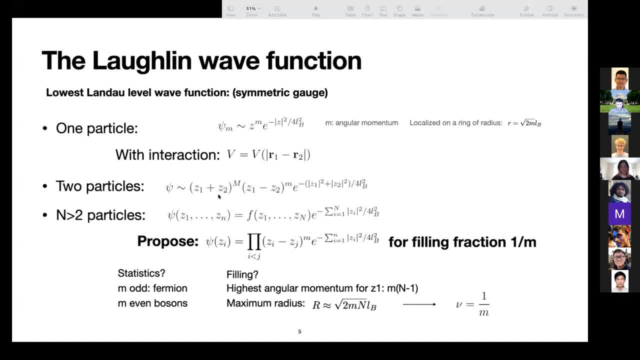 relative displacement and there and we and solving the Hamiltonia with this interaction, we can see the two particle state is actually in this form, So in general it's I mean for n equals two particles- it's impossible to solve this Hamiltonia and write down the ground state wave function. 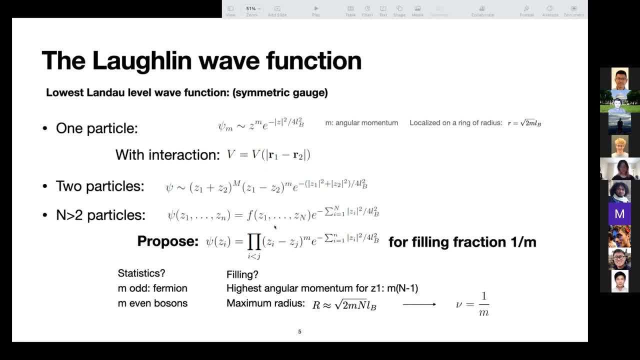 But we know that it should be of this generic form, with the holomorphic function that's, that depends on c1 to cn. If we have n particles and they should be antisymmetric, we're considering fermions, fermionic systems, So motivated by this two particle function. 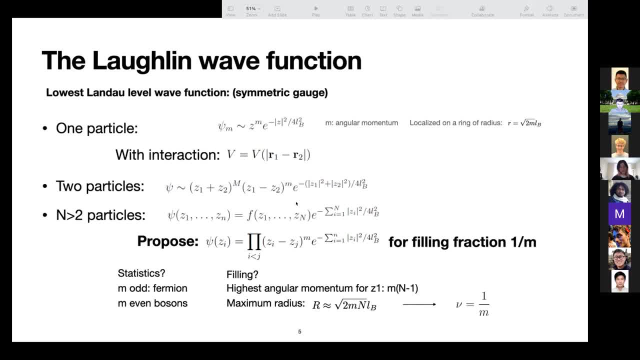 this c1 minus c2 to the n seem to be very cute, So I mean we can. so Laughlin proposed this kind of wave function for a filling fraction, one over m, fraction of quantum, whole states, Mm. Okay, So let's just. 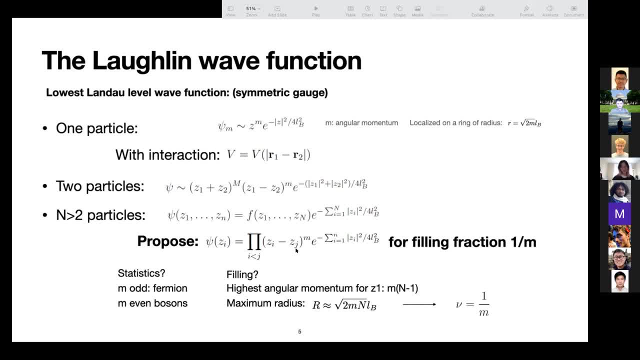 forget about the Hamiltonia for one second, for one second, and study this wave function directly: Mm. So, indeed, if m is odd, if m is odd this, this wave function, describes the fermionic systems. If m is even that's a. 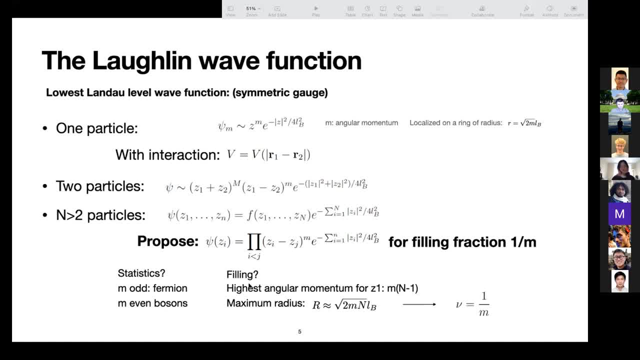 wave function for bosonic system. But how about the feeling? How do we know the feeling fraction as well over m? So note, notice that the highest angular momentum for, say, c1 is m times n minus one, where n is the total particle number. 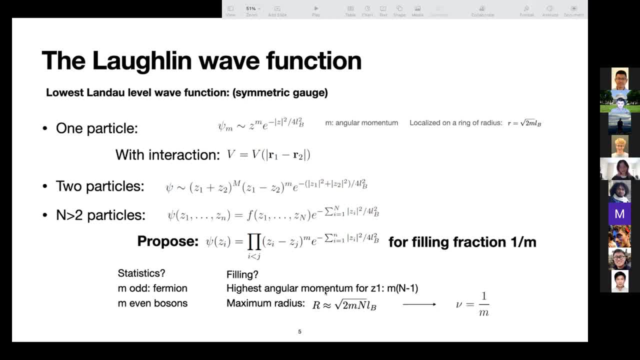 As we said before, this, this power is actually, is actually related to the ring of the radius, where the, where the part, where, where the, where the wave function has a maximum probability distribution And this, this maximum radius, can be thought of as radius for the whole. 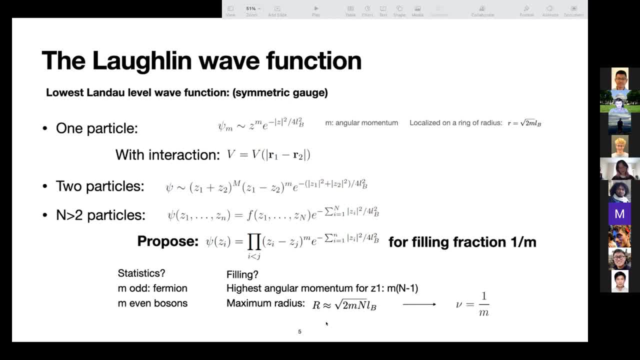 for the quantum whole droplets. It's proportional to, I mean, I mean as thermodynamic limit, where n goes to infinity. we throw out this minus one and this is the maximum radius for the whole droplet And there are and we have n particles. 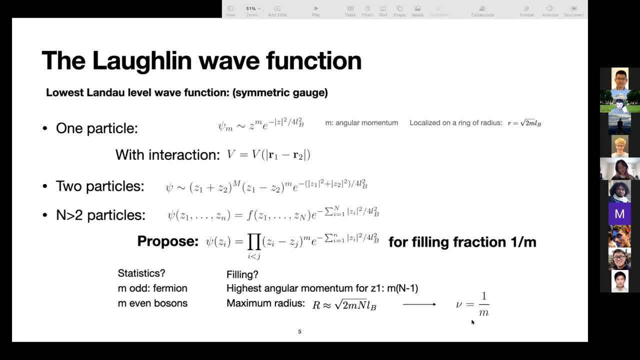 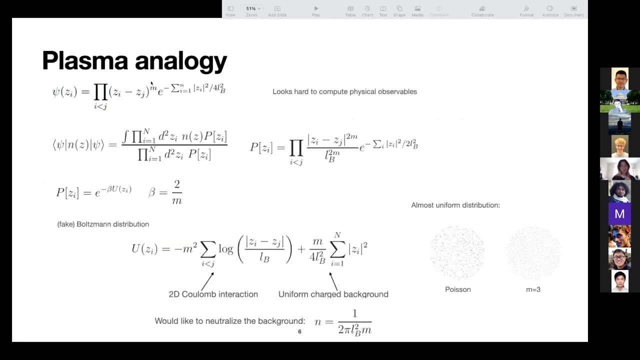 in total. So we can compute the feeling fraction of it It will give. it will simply give us one over m. So this is the, this is nice, But okay. But if we want to do anything, if we want to compute any physical observables, 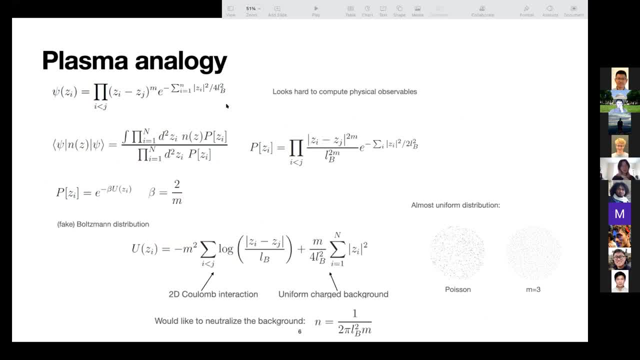 using this wave function. it seems a little bit hard because it's a many body wave function with with, with thermodynamic, with, like with many numbers of arguments. So say, if we want to compute the charge density at point C, then we need to compute something like this: 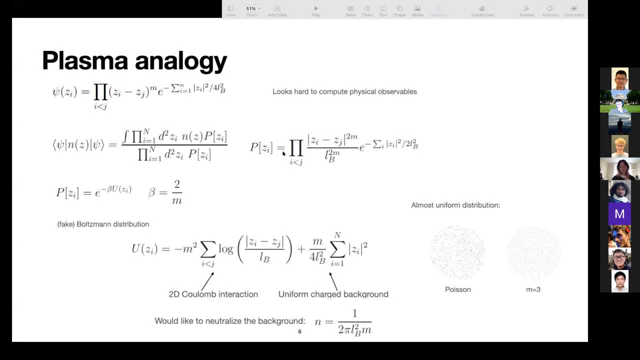 where P is the probability distribution. So, but this guy actually looks a little bit familiar. if we rewrite this probability distribution as some kind of fake Boltzmann distribution with some fake temperature, Okay, then the, then the fake potential U is, can be written. 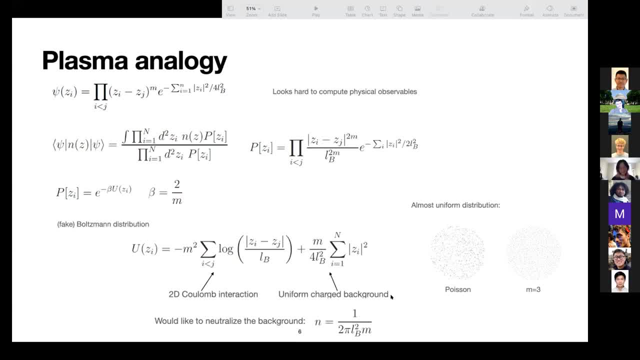 in terms of these guys. Hmm, Yeah, this, this looks a little bit this kind of looks bizarre, but if we, if. if you're familiar with a 2D Coulomb gas, then this will look very familiar to you, because actually this log term. 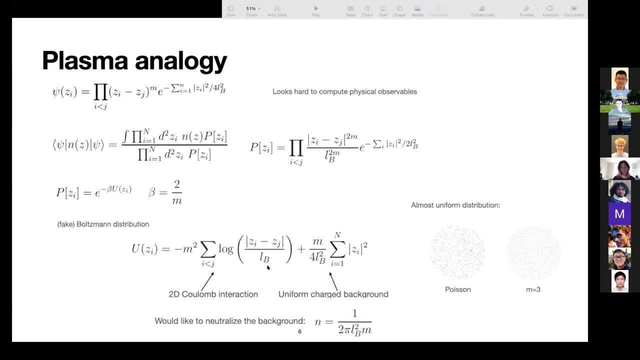 describes a 2D Coulomb interaction between two point charges, And this and this term actually describes a point charge with charge M interacting with a uniform charged background with the- yeah, a uniform charge background. So note that this M is so in this, in this. 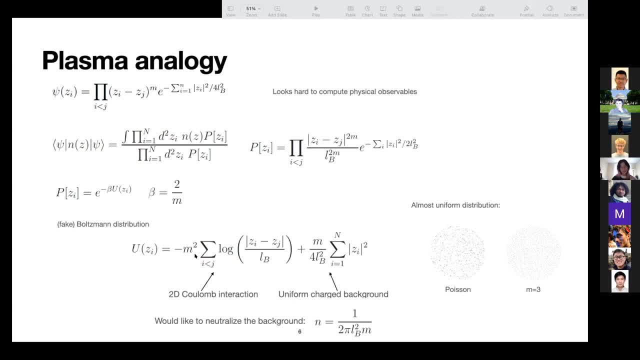 fake Boltzmann distribution point of view, this M looks like a fake charge of the particles and they live and they interact with a uniform charge background. So so, in order to have the lowest Coulomb energy, they want to neutralize the background. 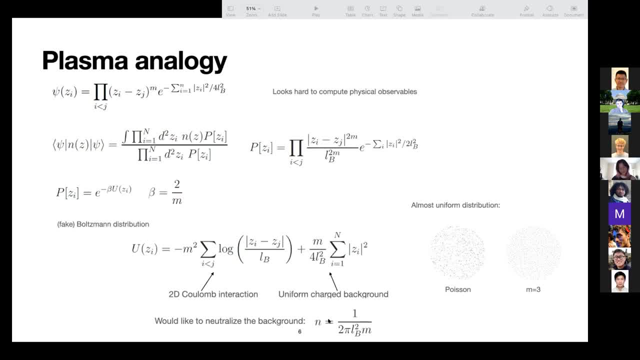 That means the, the charge density wants to be of this form. So, so, so that, so that the so that the plasma looks neutral on average, And yeah, and we can, and we can try, and we people try to plot some. this is snapshots of this. 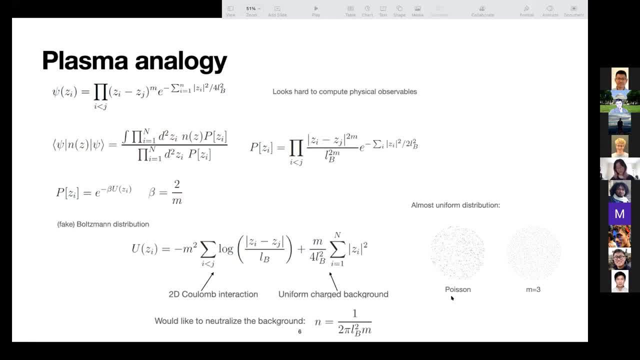 this kind of distribution. So if it's a Poisson, this uncorrelated one, that it's on the left, but for this plasma you can see that it's kind of uniform. So I mean this plasma analogy actually, I mean from the point of view of feeling fracture actually. 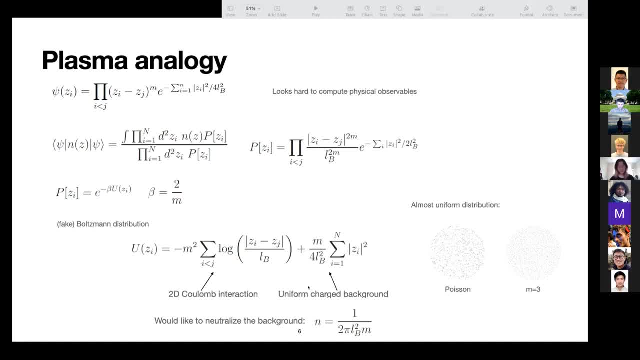 doesn't tell us anything new, But but. but it does, but it does tell us something new, as the but. what's new in this plasma analogy is that we we get almost uniform charge distribution, which seems which is not very obvious from the 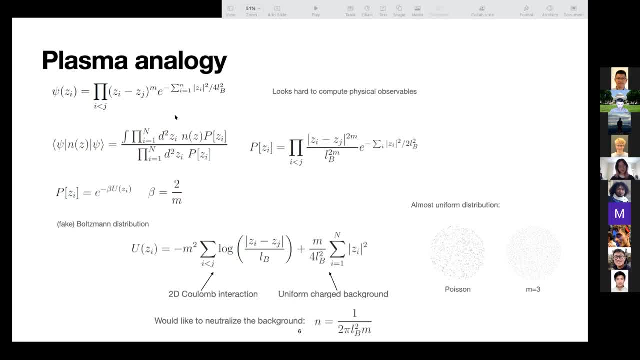 from the form of the Laughlin's wave function, because from this wave function you might think that c equals zero is some special point, but it's actually not So. so far we've only talked about the ground state, the ground state. 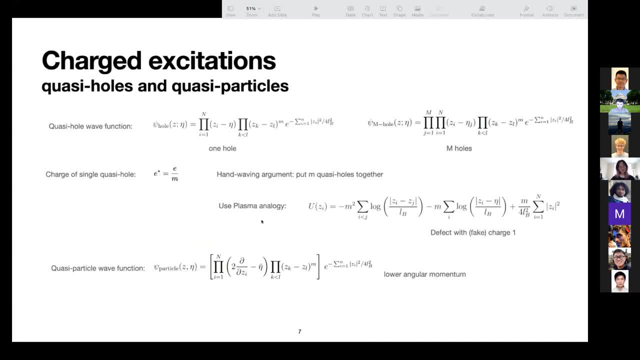 Sorry for the question, So so can you. can you then comment on, like the gauge dependence of all of this stuff that we've been doing? Is is the claim that you, even though we have this, like you know? 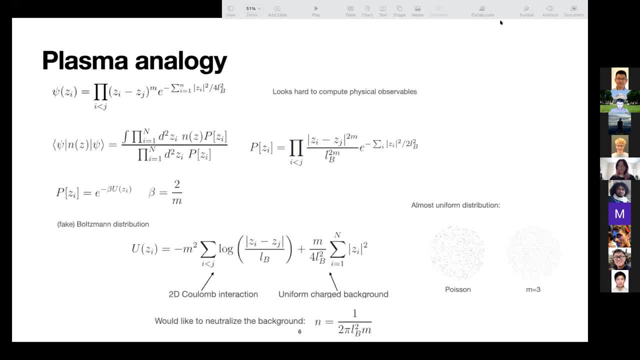 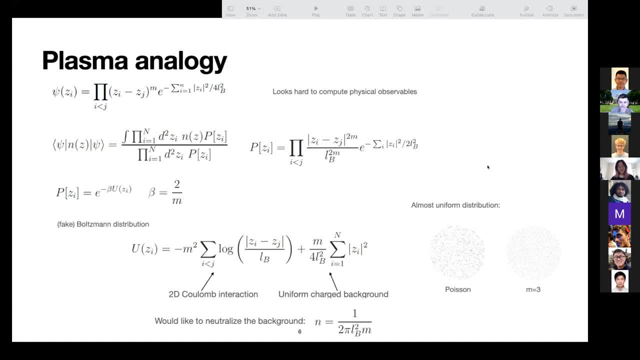 like this whole formulation depended on writing, writing, the writing, the choosing a particular gauge for the potential, Right, Yeah, Yeah, Yeah. So so here we choose symmetric gauge, right, But, but you know, if I just Well, yeah, so if I choose a different gauge, like 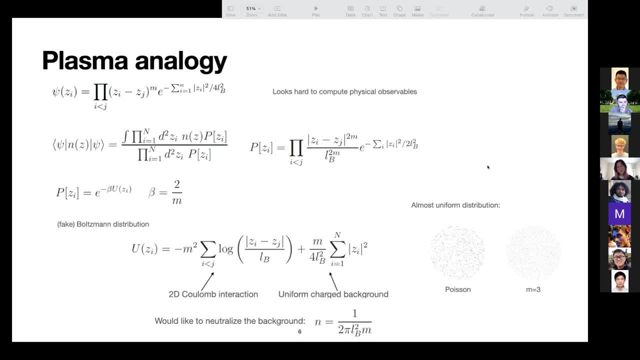 non-zero component or something. right then, yeah, yeah, certainly, and nothing is going to look like there's going to be no angular momentum, no droplets or anything so like. to what extent is the? yeah, we're, it's about the. the density of this wave function is something. 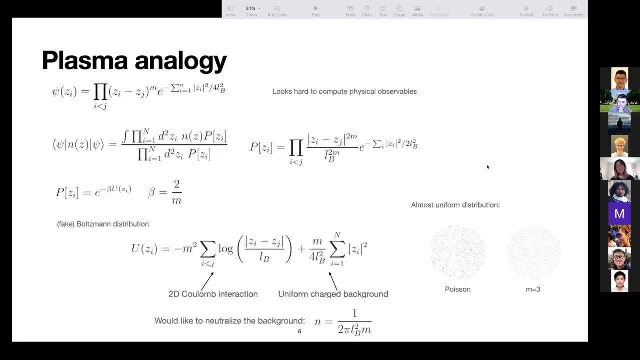 even though the wave function itself is not engaged in variant, right. what is yeah, okay, so yeah. the the so uh, yeah. but here we are actually computing a gauge, invariant quantity. right, it's the uh charge distribution, so it doesn't depend on our gauge choice. i mean the uh, i think the uh. 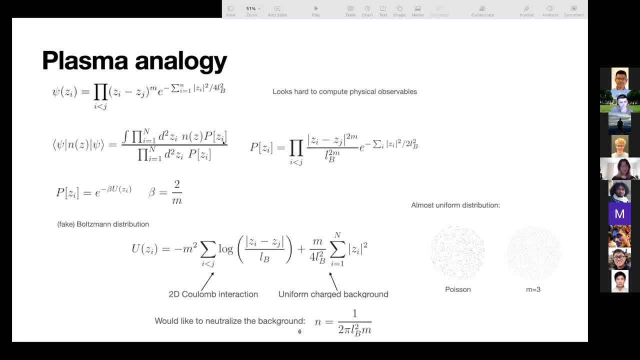 the, the, the. the Beauty here is just that I can choose the convenient gauge such that I can see the results in a very easy way. Yeah, instead of say choosing, choose a Landau gauge where I don't know how to write this wave function will be a little bit complicated. 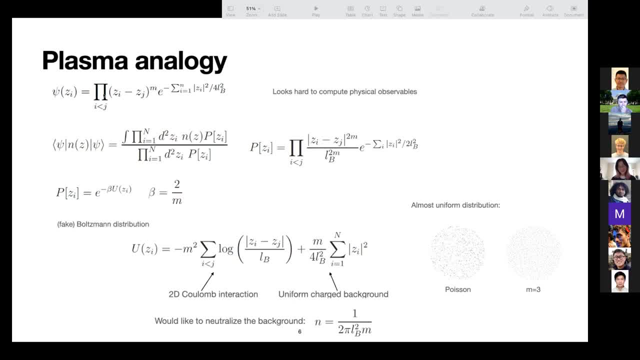 Wait, sorry, this is just dumb, but can you remind me why this is? Why is the expectation value of n in that particular psi is independent of the formula, Because our gauge transformations aren't like acting as phases on psi or anything. I'm just thinking to myself that the form 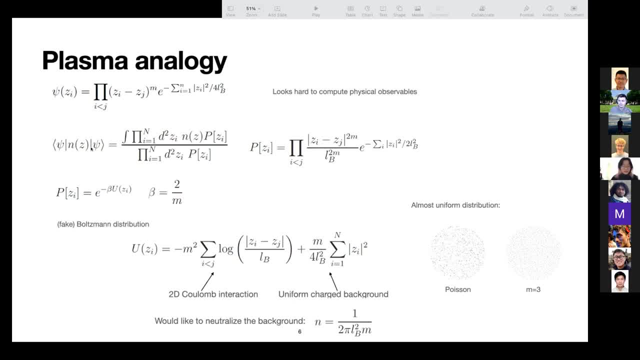 for the wave functions would look like completely different in that, Yeah, in a different gauge, right, Yeah, Yeah. but n here is just some. I mean it's just a delta function. I mean this is a physical observable. 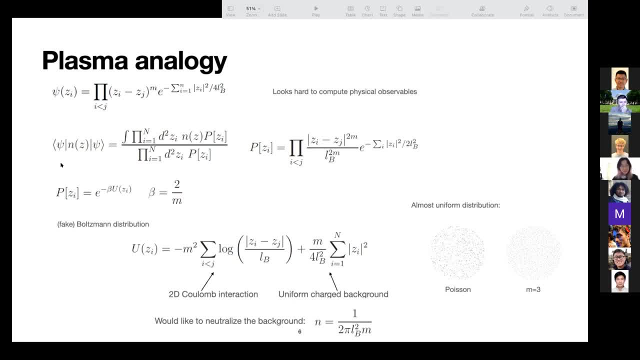 It shouldn't depend. It shouldn't depend on any gauge choice. Yeah, and this plasma analogy, just I mean it's an intuitive way to see how this to I mean to have an intuition for the property of the wave function. 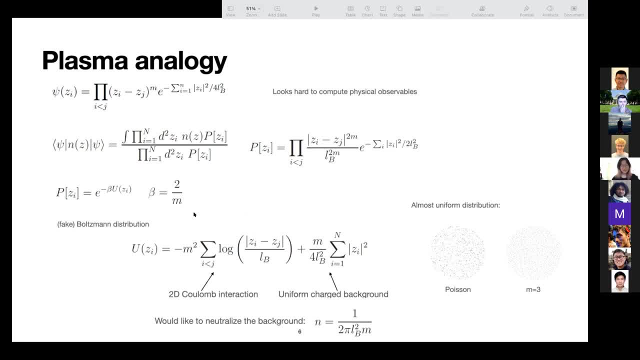 I mean it's not there's. no, actually, there's not actually a temperature. I mean it's not a temperature or something, Right, okay, so even though the whole wave function is localized in an exponentially localized in a droplet, 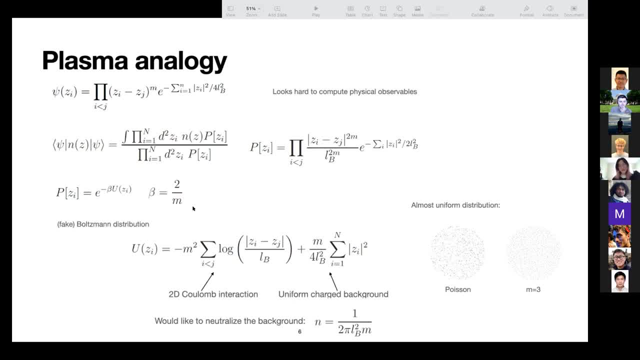 the claim is that the density is still uniform. Yeah, yeah, the density is almost uniform. But isn't that weird that, since psi only has like is exponentially, is only supported on like a compact region, Okay, well, whatever, Okay, I guess it's just writing for those. 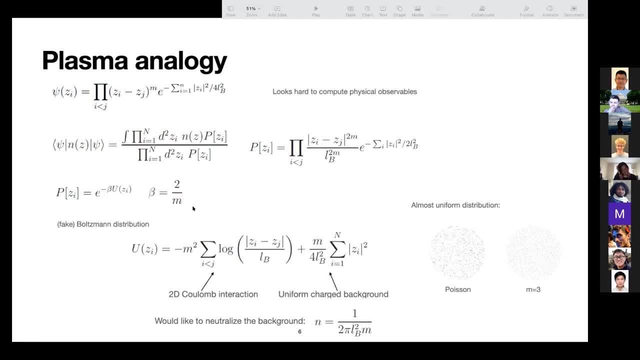 Yeah, that's, I mean that's. I agree that's very counter intuitive. Yeah, but if you think of it in this plasma way, it seems, it also seems a natural conclusion. I mean it's not. I mean it's not at all obvious. 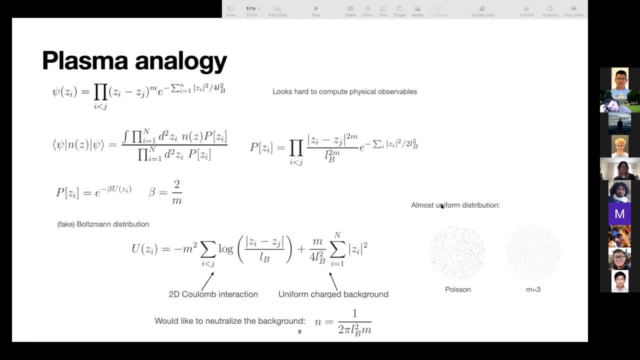 from the form of the wave function. I agree, Yeah, and so I also need to be careful about the. you know, Yeah, and so I also need to be careful about the. you know about this plasma analogy, because here it's actually a finite temperature. 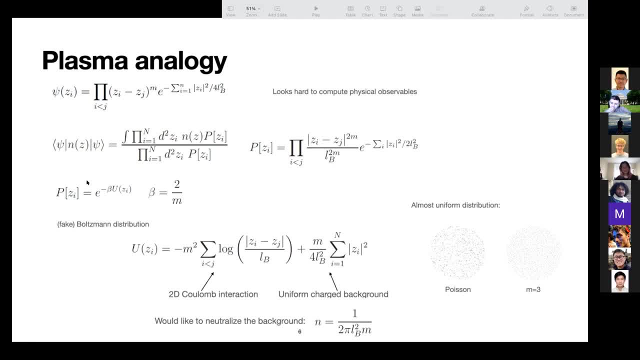 And yeah, so one may worry about whether this guy, whether this charge, will froze stuff like that. Yeah, but if one do, the people did numeric on these stuff and found that for M, say, less than 70 or something. this uniform distribution picture. 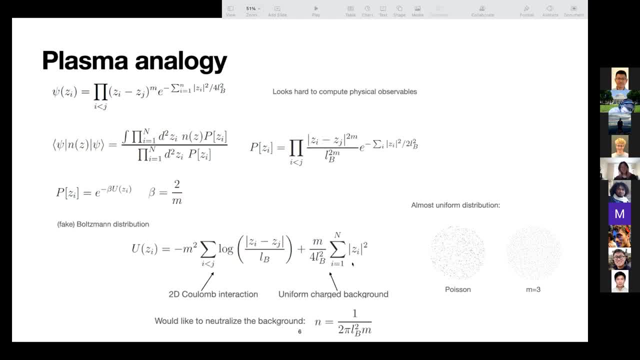 actually works pretty well. Yeah, okay, Oh, go ahead. Sorry, any other questions? No, I was just saying maybe I'm being stupid here, but it being localized to like to a ring. that was with the wave function, right? 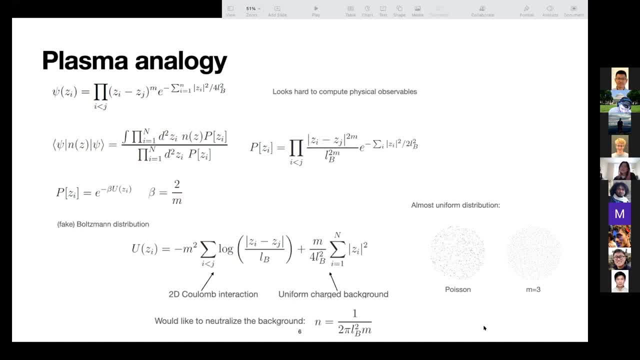 So if you were looking for some place for gauge dependence to rear its ugly head, I mean, that's probably where I would look. Once you look at the charge density here, that's where you applying a plasma analogy, right, Yeah, Right, so I would trust the plasma analogy. 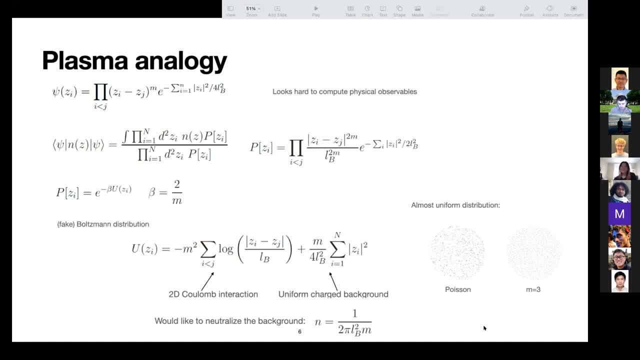 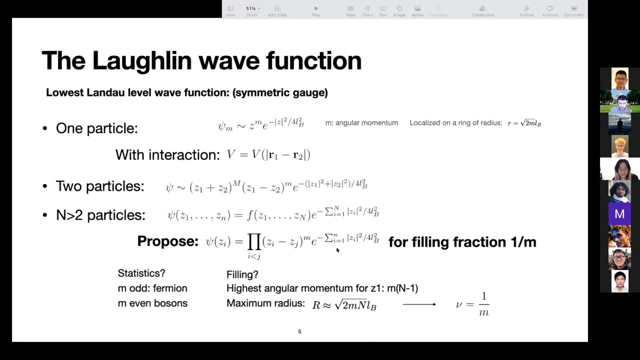 more than the wave function being localized on that ring, At least when I'm thinking about gauge dependence. Anyway, sorry, unnecessary comment. Yeah, yeah, Sorry, right right Here in the previous slide I just gave a very hand wavy argument. 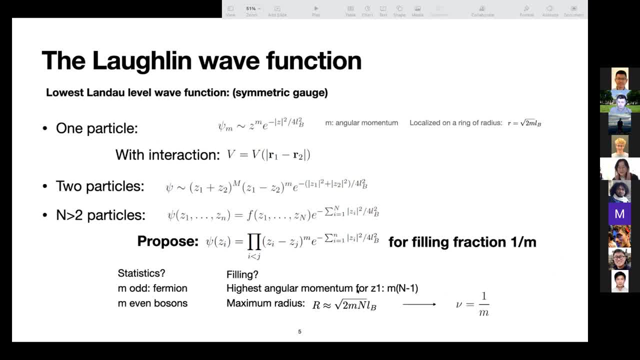 and it's actually only for one single particle It's. I mean, after all, we're dealing with this. If I send magnitude of Z to be very, very large in the thermodynamic limit or something, it still looks like psi goes to zero. 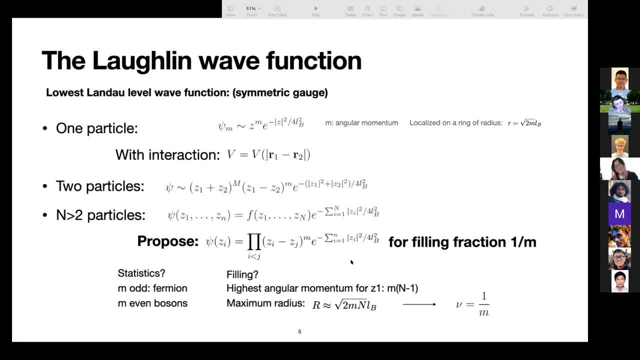 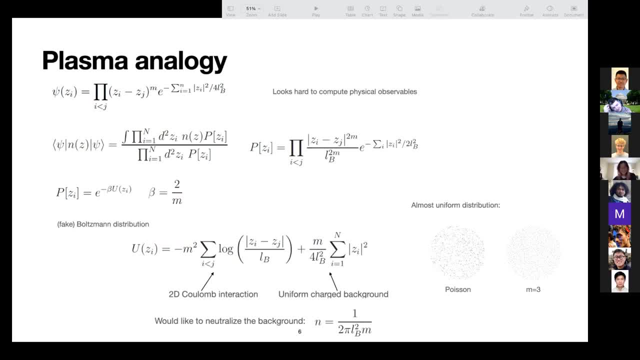 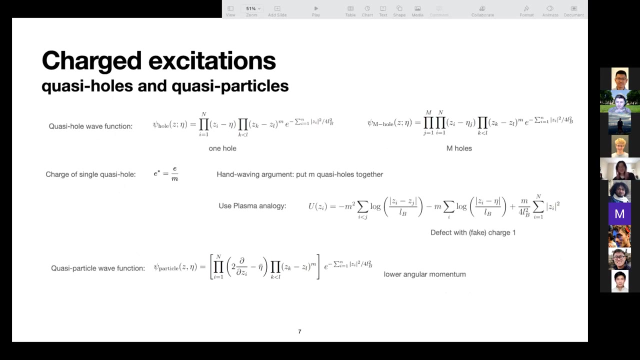 It's too fast for it to be able to provide a uniform. Well, anyway, Okay, yeah, Right. so far we've only talked about ground state, So let's consider what kind of excitations we can have. So we'll be talking about charge excitations first. 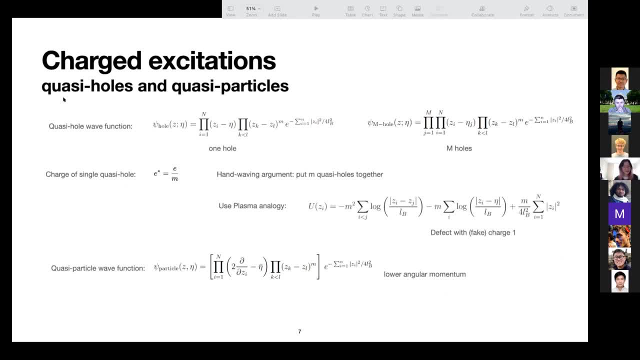 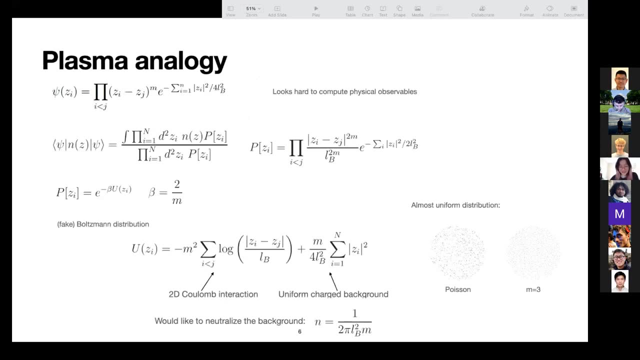 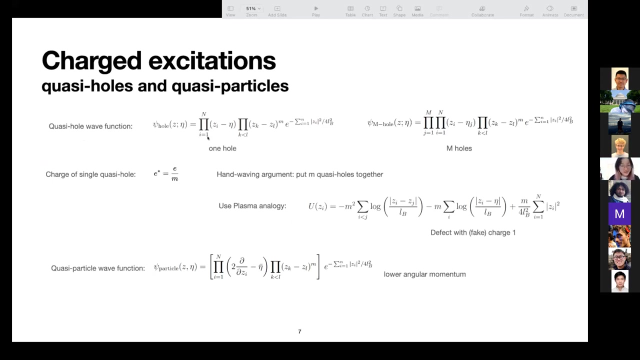 So that means we are talking about quasi holes and the quasi particles. So I mean. so, in the spirit of guessing wave function, we can just guess the quasi whole wave function. So so yeah. So people propose this guy to be a wave function of one whole at position eta. 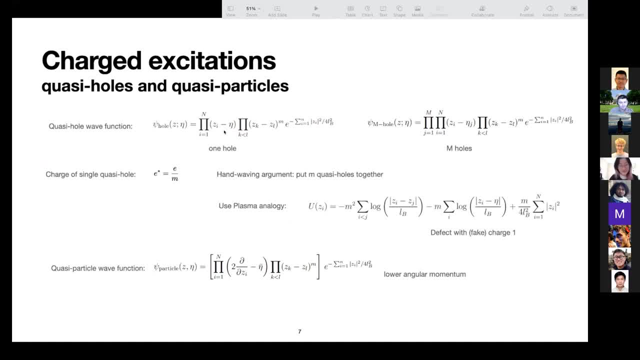 So let's see if, if this is, I mean if, if this makes sense, So if I have one whole at position eta, I mean this wave function does, does, does, does not, does not. I mean it is, it is not, it does not, it does not work. 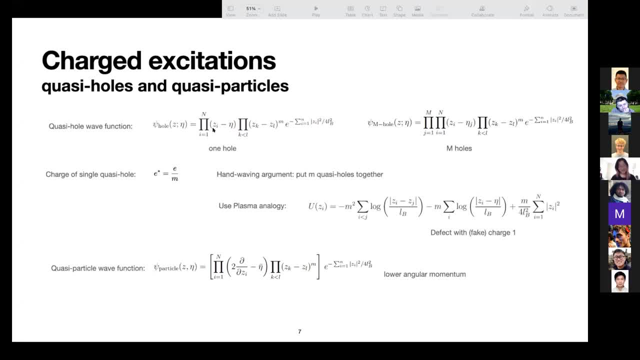 it does have vanishing amplitude when Z approaching eta. So it looks fine, And we can also try to put M holes at position eta one to eta M. So yeah, this seems to be legitimate. So let's see then. how about the charge? 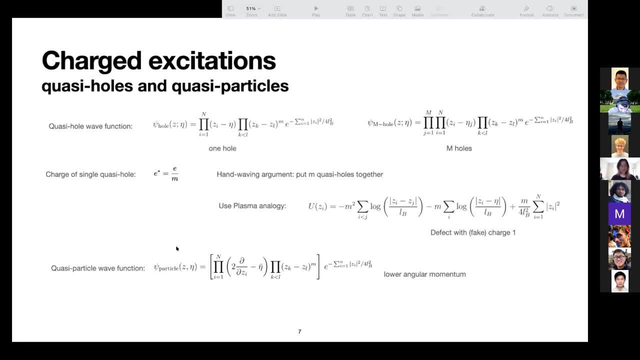 of a single quasi-hole. Surprisingly, the charge is actually one over M. Okay, so I can. one hand-waving argument is that if I put M quasi-hole together and they all at position eta, then this guy is going to be M. 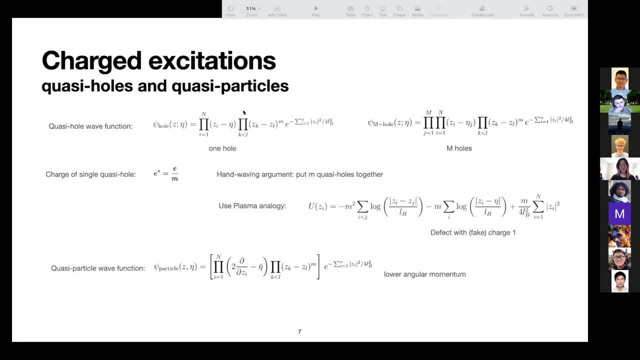 This guy will just be Z minus eta to the power of M. It looks like the Laughlin wave function we get before, but with eta fixed instead of varying. So that means we fix one electron in our system. So yeah, so that means if we put 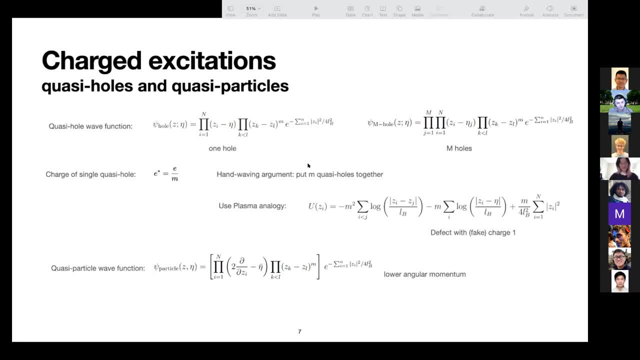 M hole together, we get an electron. Yeah, that means the quasi-hole actually has a charge, one over M. Yeah, this may not look very convincing, but again we can use the plasma analogy we just learned and write the fake potential, which looks like this guy. 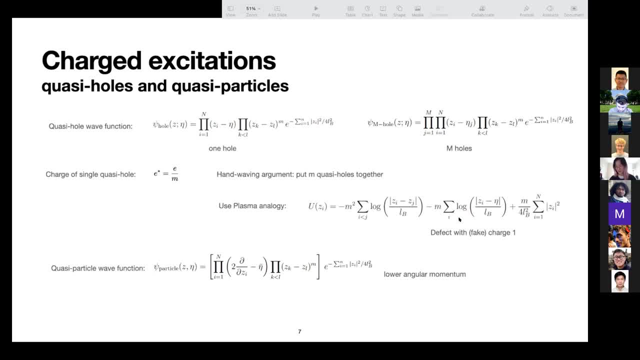 So for this one-hole function, one-hole wave function, we get additional term which looks like this: It's a defect with charge one. So, right, as we said before, the whole purpose of this plasma is want to be neutral. 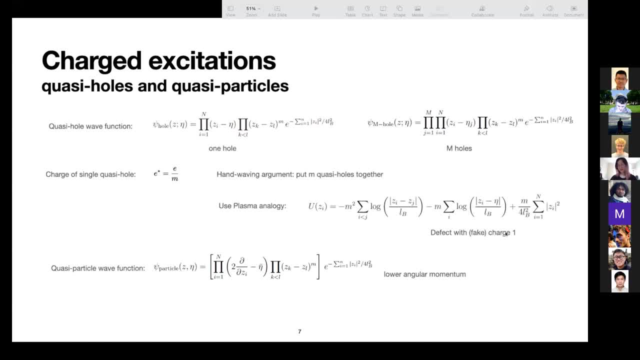 So if I have a defect with charge one, then then all the particles will want to come to this, want to screen this fake charge. But notice that in this plasma analogy the charge of the particle is actually M, So I only need one over M of the charge density. 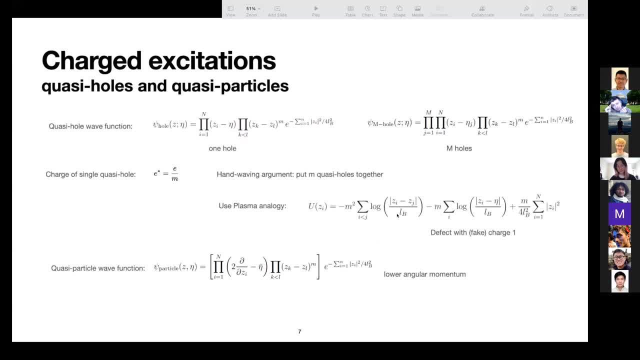 So but yeah, but the particle actually has physical charge E, So that means the. that means the charge of the quasi-hole is one over M times the physical charge, So we can also consider a quasi-particle wave function. One way to consider quasi-particle wave function is that. 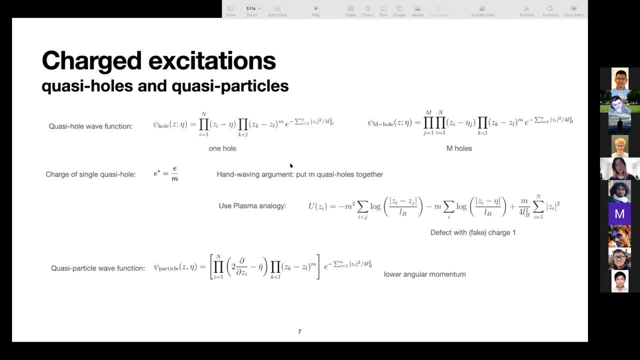 So notice that in the quasi-hole wave function we want to a ray on raise the power of angular momentum such that the quantum hole droplet will be larger, but we still have n particles, so it will be so effectively it will introduce hole If we 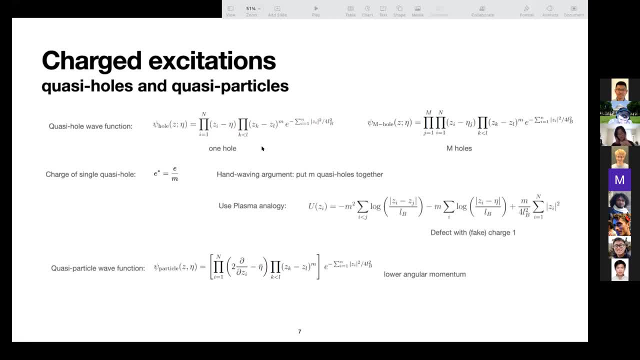 want to introduce particle, that means we want to lower the angular momentum. So one way to do that is, of course, we can divide this guy by itself once, but then it's problematic because it will introduce singularity. Yeah, but, yeah. but we can also multiple multiply this guy by z bar. that will also lower the angular 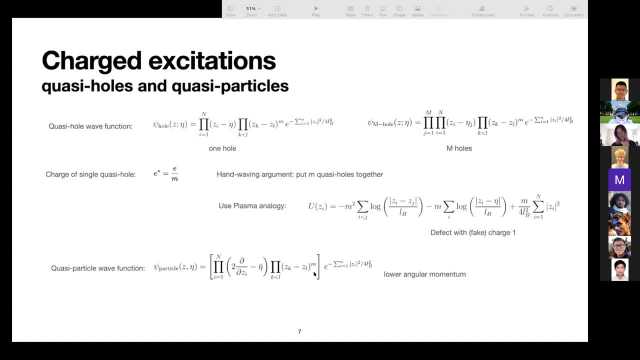 momentum. but z bar is not legitimate, a legitimate lowest Landau level wave function. So people did some projection to get this form of quasi-particle wave function. I mean, it looks very hard to deal with And yeah, and indeed I'm not going to talk about this wave function anymore. 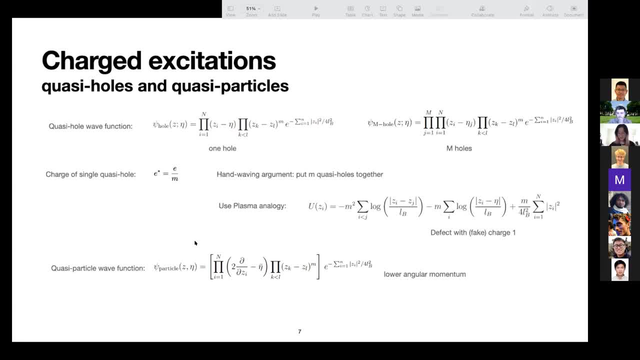 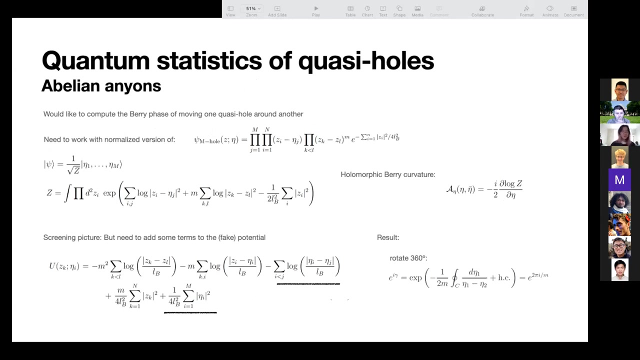 I'll be dealing with the quasi-hole wave functions. So yeah, so I told you that the quasi, the charge of a single quasi-hole, is one over m, But how about the quantum statistics of these guys? So that means, if I exchange two quasi-holes, 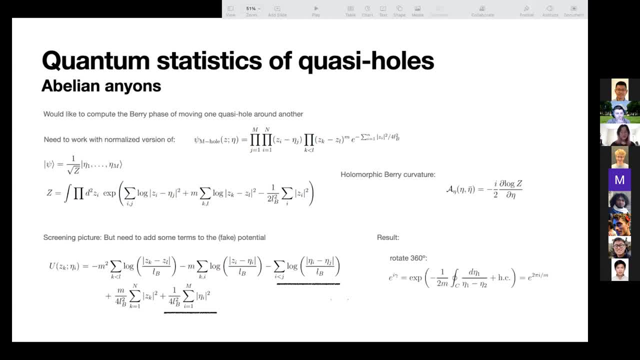 what will I get? Yeah, so we can. we can compute this exchange angle by considering the Bayeric curvature of this wave function containing m holes. and you know, just move one hole around another one to get to the statistic angle. But caveat is that in order to compute the barrier curvature, 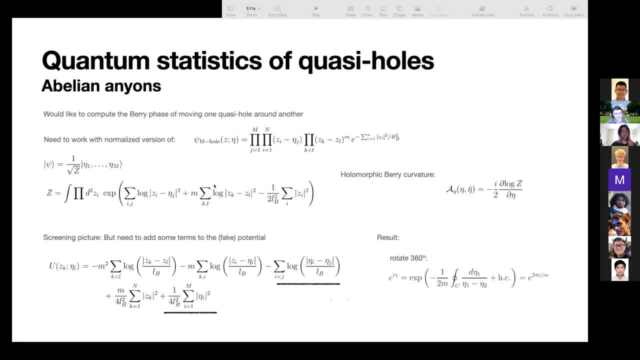 need to work with a normalized version of this guy, which which is? which is this one where c is just this partition function. we get in the plasma analogy, yeah and right. again we want to use, again, we want to see what a plasma analogy can teach us. so 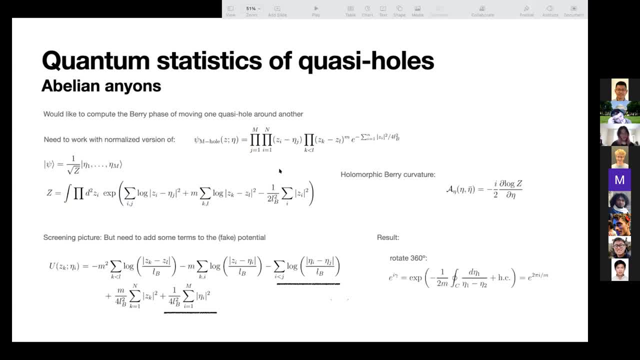 so this whole systems looks like we have some kind of defects and also a uniform background charge and the coulomb interaction between particles. there's a coulomb interaction between particles, coulomb interaction between particle and defects and a coulomb interaction between particle and charged background, but that's not the 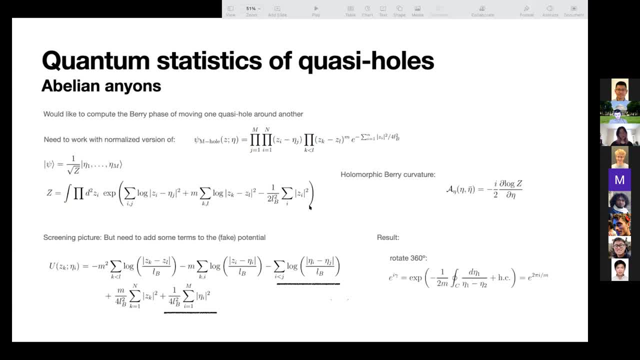 whole coulomb interaction. if we, if we're considering a system with with those charge defects, we are missing two terms. one term is the coulomb interaction between the defects themselves, the other one interaction between defects and the charged background. so if we add those two terms, uh, 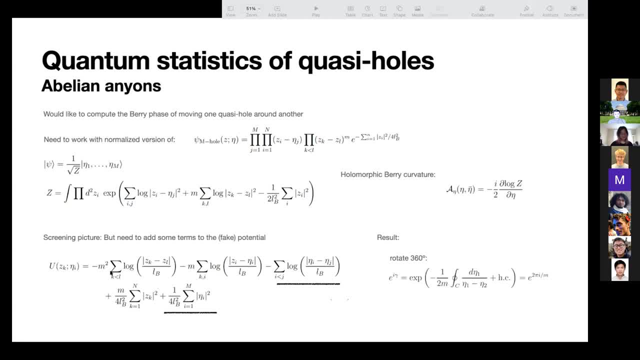 looks like uh, it looks like so. so this, this uh corrected uh potential, actually describes uh, this actually describes the uh interaction, the whole column and interaction energy, uh containing these defects. so uh, yeah, so uh. as i said before, the whole purpose of the, the plasma is, is that they, they want to be neutral. so 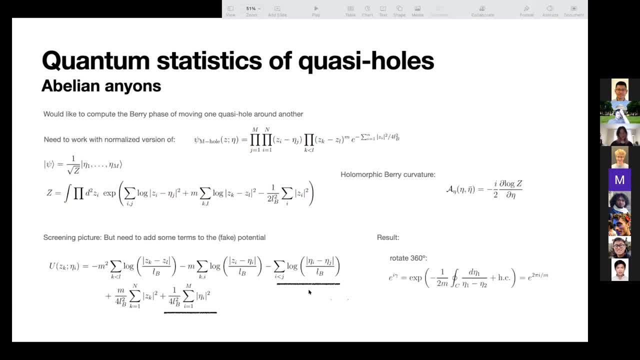 yes, so if, if the uh, if the plus, if the total stuff is neutral, then it doesn't matter where i uh, it doesn't matter where i put those defects, it will, they will be screened. so with that means, uh, actually, if we consider this, this corrected potential, 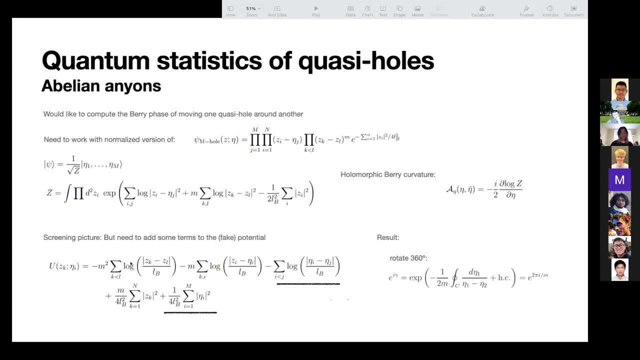 if we replace this corrected potential, uh, replace the original potential by the corrected one, uh, the resulting part, the resulting fake partition function will not be no well, very. it doesn't depend on the position of add-up. so that means the the barrier, the barricadrature of of this guy actually vanishes. 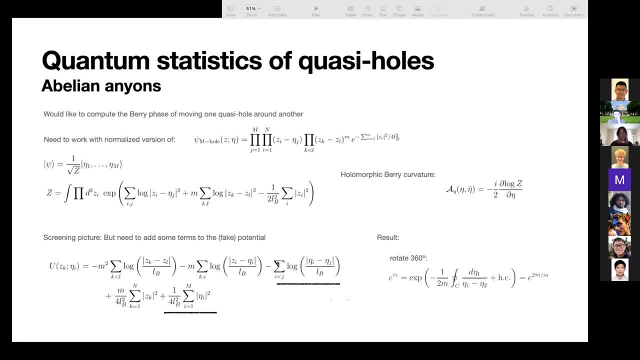 so we only need to consider the, the effect of this, these two underlined term, to the barry curvature. yeah, this is uh much. this is much easier to deal with because they, because we don't need to integrate over the the in a very thin layer or we are simply going to library to Mark 7-y tonight. 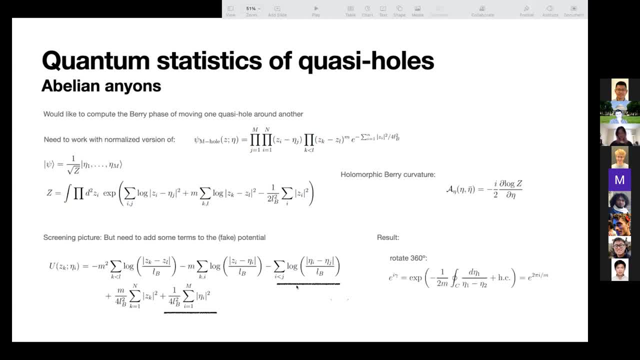 those c's and indeed we. if we compute the holomorphic barrier curvature of this guy, we get some factor like this. so if we uh rotate, say one quasi whole around the other. rotate, say eta one around eta two, we'll get a phase factor that's proportional to uh two pi over. 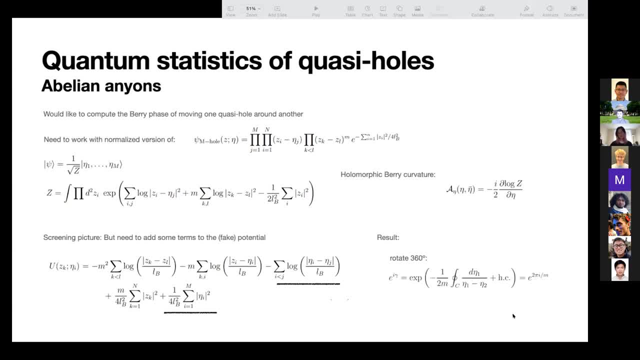 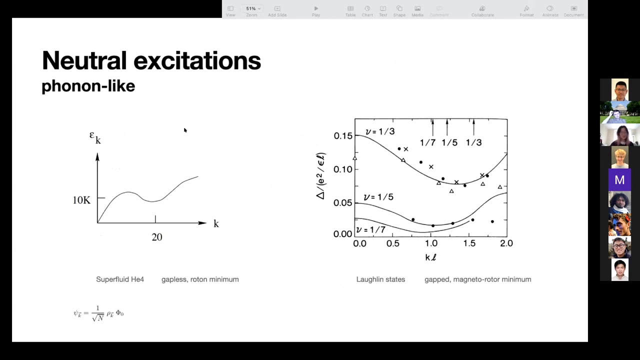 m, and note that the statistic angle is actually rotate 180 degrees, not not two pi. so the statistic angle is uh, one over m, so uh, yeah, okay, uh, so, uh. so so far we've been dealing with a charged excitation. i also want to mention, in bypass, we uh, in those, uh, in those systems, there's also a neutral excitations which are 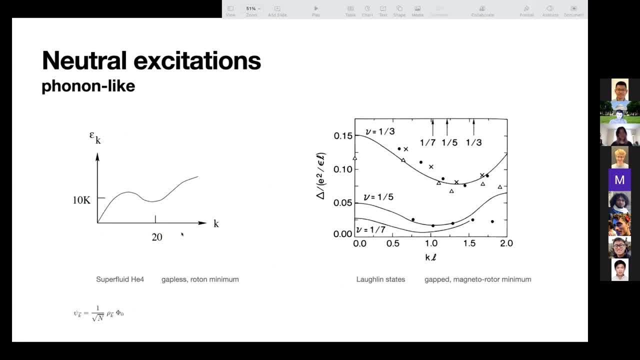 funnel. like it comes from uh density fluctuations. it's similar to uh what happens in superfluid helium-4. but a major difference between the uh superfluid and the quantum hall fluid is that the uh, the phonon distribution is the phonon is gapless in superfluid, but it's uh gapped in a quantum hall system. 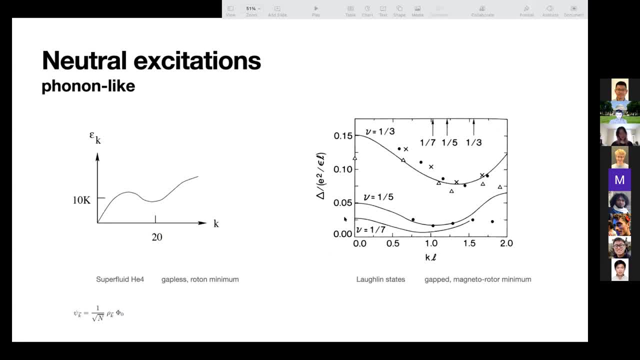 because in superfluid there's a ghost tone mode. but uh, but this quantum whole fluid, actually it doesn't have any ghost tone mode, etc. and uh, analogously, there's also a roton minimum in this, uh, in the quantum whole fluid, which people call a magneto roton minimum. 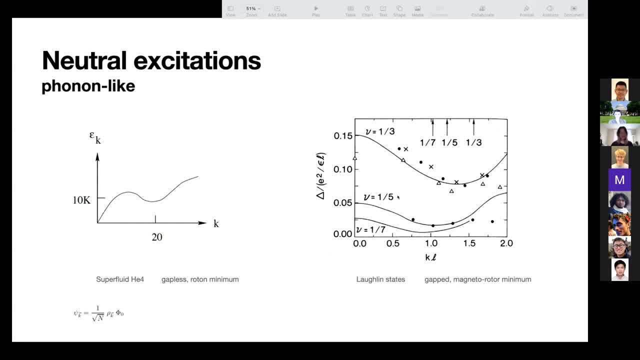 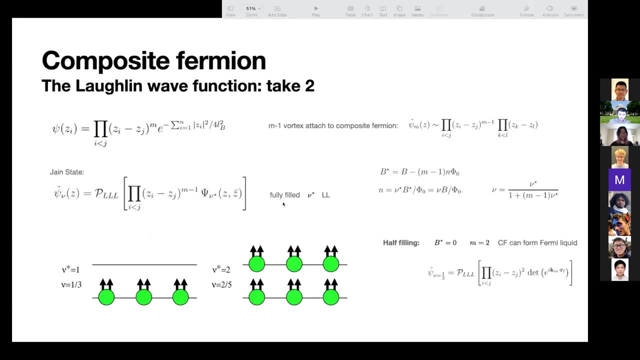 yeah, if, yeah, if i have, if i have time, i can talk about how to get this uh more. but uh, yeah, let me just skip the neutral excitations. okay, so far we talk about a lovely wave function and the plasma analogy to it, but uh, uh, actually we 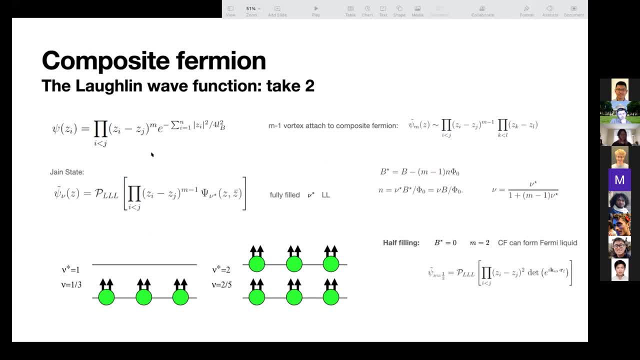 can view a lovely wave function from from another point of view, which is the point of view of composite fermion. how does this work? uh, work. So the Laughlin wave function is this guy. And if we decompose this factor to m plus 1, power of m plus 1 and 1, this second guy looks like n times this exponential coefficient. 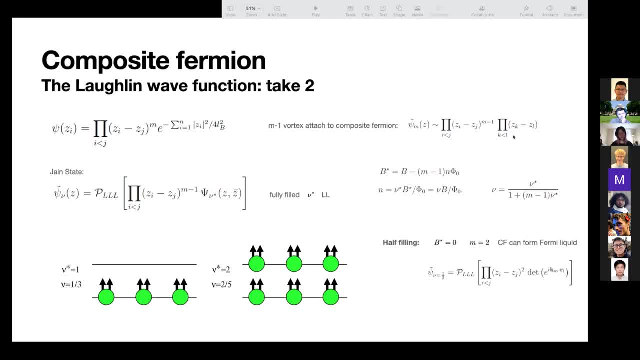 and it just looks like a fully filled lower strong dot level wave function. So, but I mean intuitively, this Laughlin wave function just looks like we attach to this z another vortex of power, m minus 1.. So this motivates Jane to write down some. 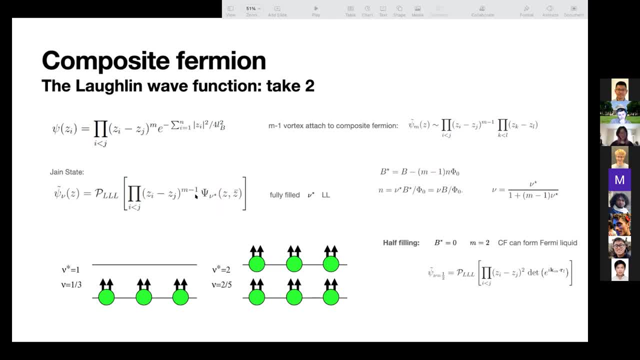 states Like this guy, where this new star is a wave function of a fully filled new star's lower dot level. In the case of Laughlin wave function, this new star is 1. And attach to it some m minus 1 flux And after that we need to project the whole thing back to the lowest. 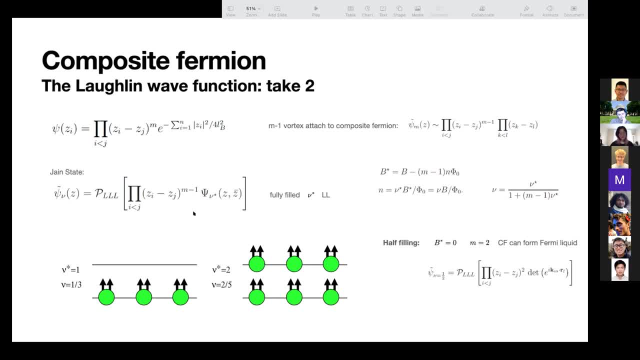 one, Because in this fully filled, if new star is not 1, there will be some anti-holomorphic part that's not allowed for a wave function in lower strong dot level. Okay, So let's see what this composite for. by the way, we call this, we call the Fermi. 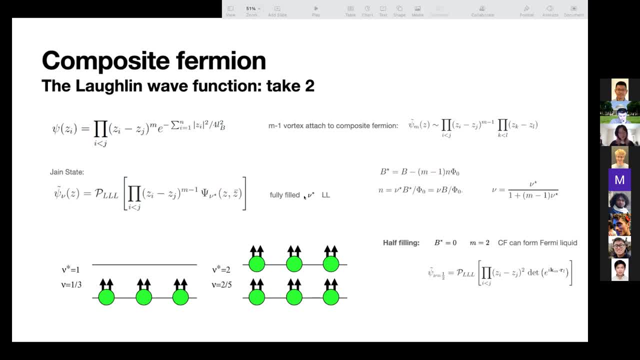 because Fermi in this new, in this new star of the composite Fermi. So let's see what this composite Fermi perfectly can teach us. yeah, so this. so, first of all, this new star, the fermion, the fermion inside this, this, this landau level. 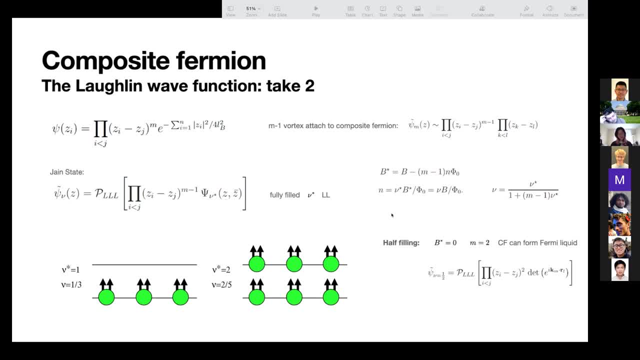 wave function, it should feel a different magnetic field because we attach vortex to to it to get to get back the original one. so yeah, so actually the magnetic field, magnetic field felt by the composite fermion as the original magnetic field, minus the m, plus one which is the stress of the 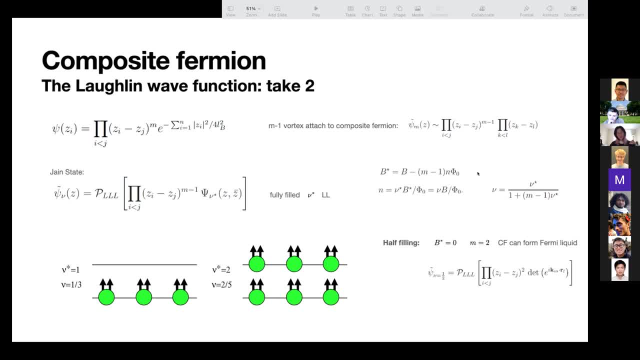 vortex times the like the density, density of those gas. so and also the. for each composite fermion we attach m minus one vortex. so the charge, so the particle density of the composite fermion and the particle density of the original guy should be the same. that allows us to determine. 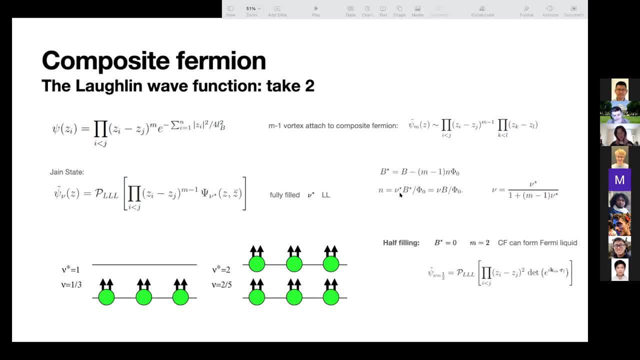 a new feeling fraction, which is this new star and related to the original one. so, yeah, so the relationship between the new star and new looks like this guy. um, we can pick any new as well, as it's an integer. so this gives a and an m is also an integer. 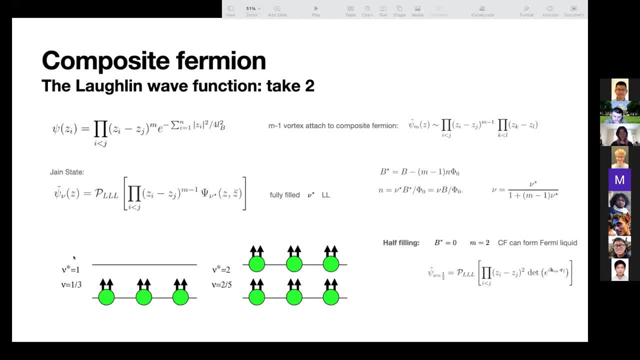 so this gives gives a whole sequence of wave functions which are called uh, which is called jane, c, jane sequence. so we can look at some examples. for example, if, if we, if we attach uh to say m equals three, that means we attach two vortex to and to a fully filled uh. 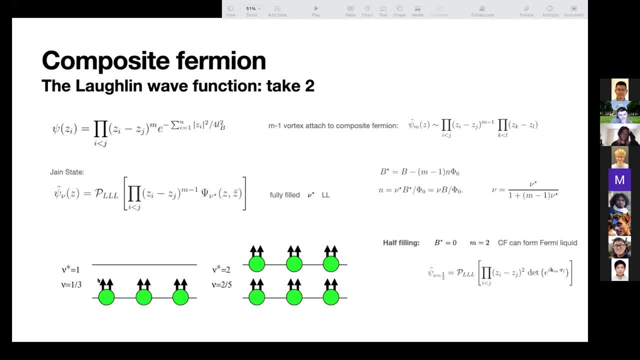 zeros, for if your first level, new star, equals one a zero, so so we'll get to new equals, uh, one over three, which is the which is which indeed gives the uh right feeling factor because, uh, remember, for the loveling state, if we we have the feeling pressure, we have to. 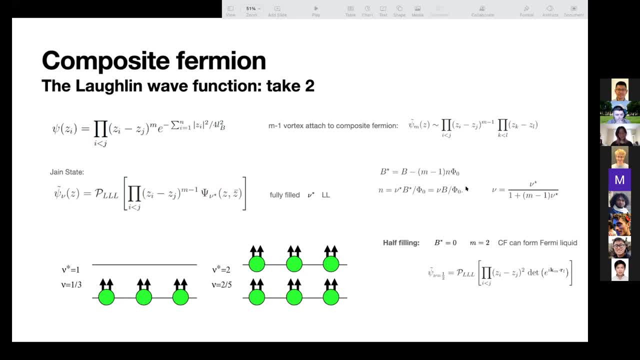 pressure one over M, And this can also be reproduced by this, by considering composite fermion. Yeah, actually, there's a very interesting example to it is if we consider M equals two and this B star equals zero, that will give a half filled Landau level. 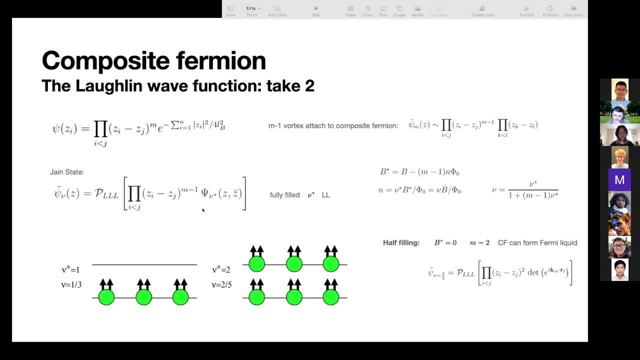 But notice that this wave function is actually not correct for that half filled Landau level because the magnetic field of the magnetic field that's filled by the composite fermion is actually zero. So the composite fermion can form liquid. So we can. 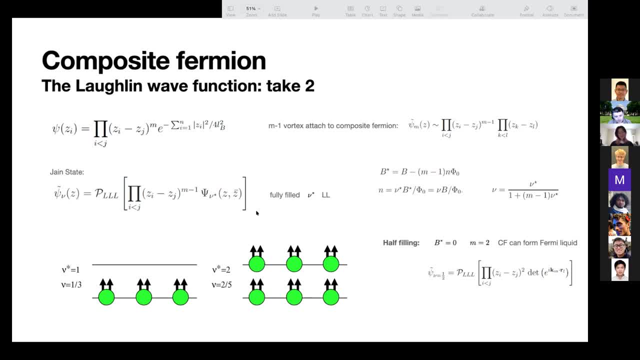 so instead of this chain state we can write a new equals half state, like this guy, where this determinant is just a wave function of a Fermi liquid. Okay, that's good. Another question: So I sorry, I just can you remember? 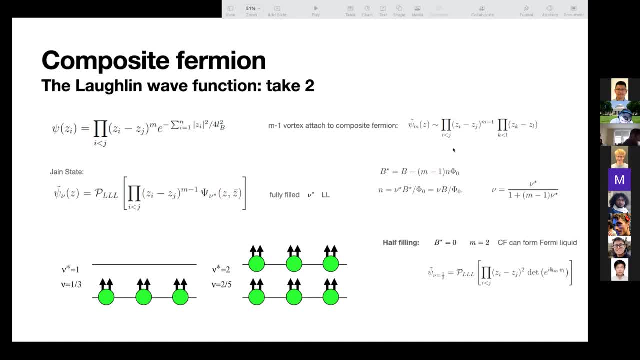 remind me why the lowest Landau level has no Z bars? Oh it just. it just comes from the symmetric gauge. If you choose a symmetric gauge, then the lowest Landau level, the lowest Landau wave function, will always be a whole homomorphic function. 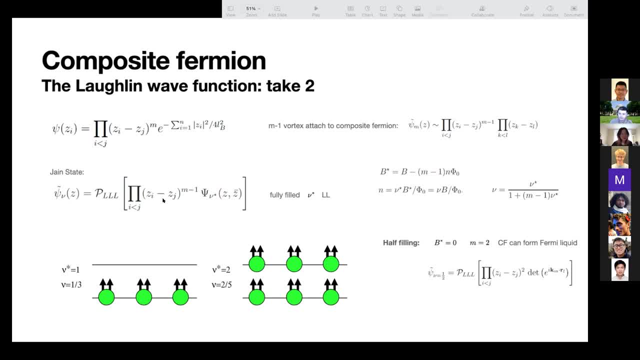 times some coefficient. Oh, here I just. I mean, here I didn't include any the exponential factors, But okay, So that follows from the Hamiltonian or something, And that boils down to, so, first of all, the energy scale in our problem. 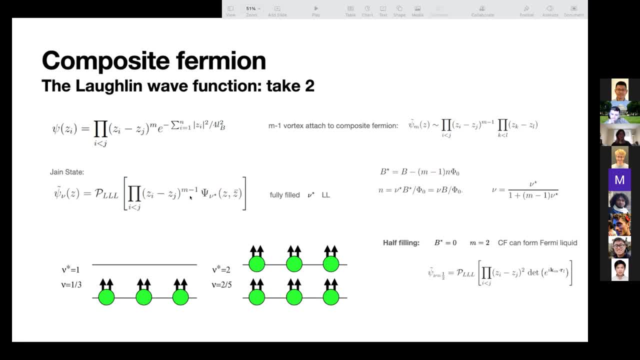 is the coulomb energy much less than the London level splitting. So we can just consider the projected Helmer space spent by the wave function of the lowest London level of the non-interacting Hamiltonian. Yeah, okay, And so the claim is that if I were to write a Z bar, 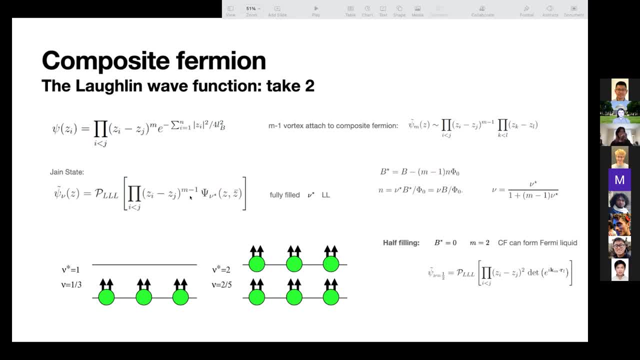 inside or something. what would that be doing? If you do, if you do a projection to the lowest London level, it will give you something like partial Z Uh-huh. Okay, so the rule for do this P-L-L-L thing right? 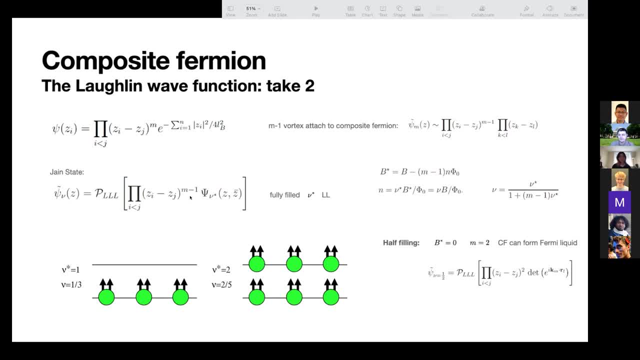 If I have some Z bars in psi, I try to replace them with derivatives, as you did earlier when you were describing the quasiparticle wave function. Yeah, yeah, yeah With, yeah, with derivatives on the, on this, on this factor. 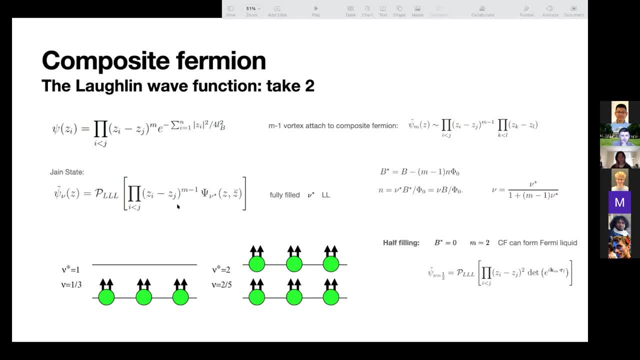 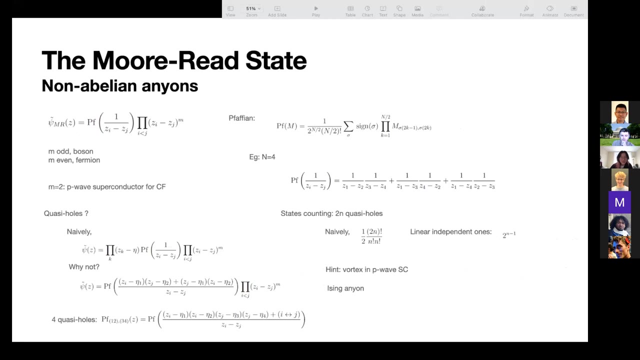 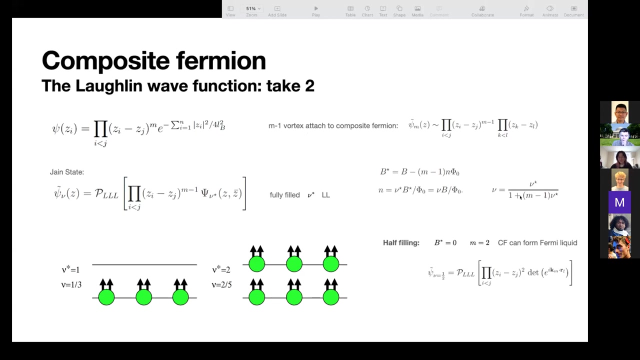 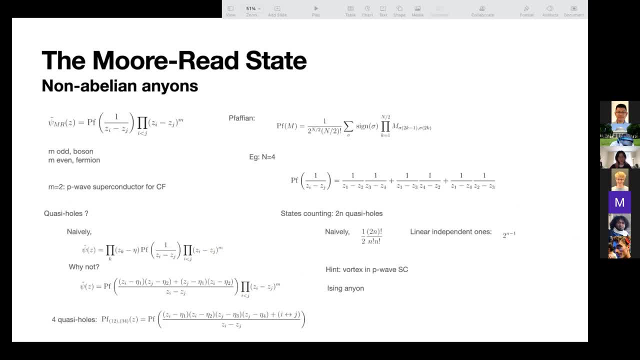 the motion, And so, in the spirit of guessing constant wave function, we can try to do more, more than a Loefflin wave function. So, yeah, that is more. I really propose this, these, this kind of this kind of states. 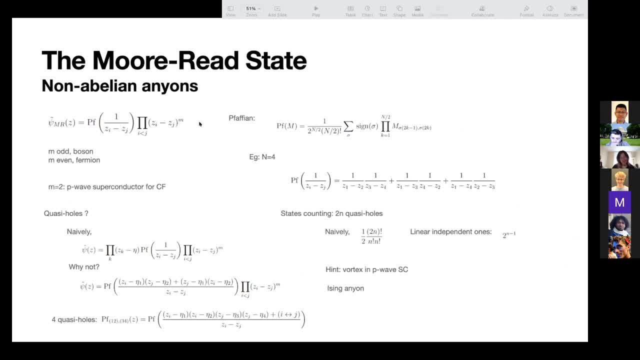 So this: I ignored the exponential factor, so the exponential factor is not binary. So that gave me the fact that at this level of phi, of this process, So this small read state has a very peculiar form, with a phaphia in front of it, so it's also called phaphian state. 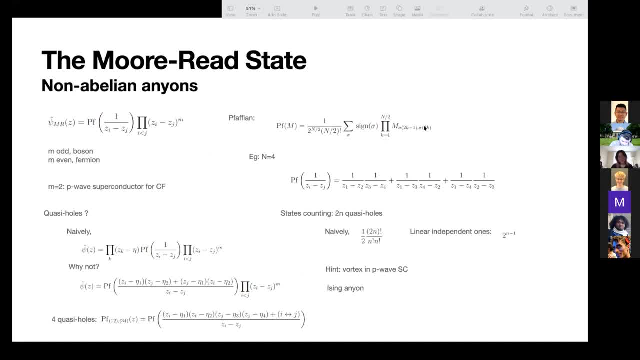 So the phaphia is something like a square root of determinant, which is defined by this expression. So yeah, so let's first look at a single example. if we have n equals four, So the phaphia of this guy with four particles can be written as something here: 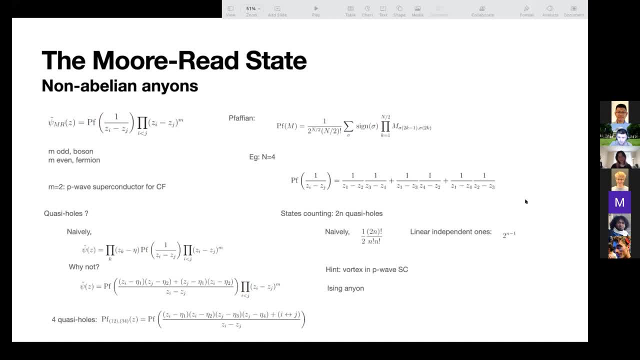 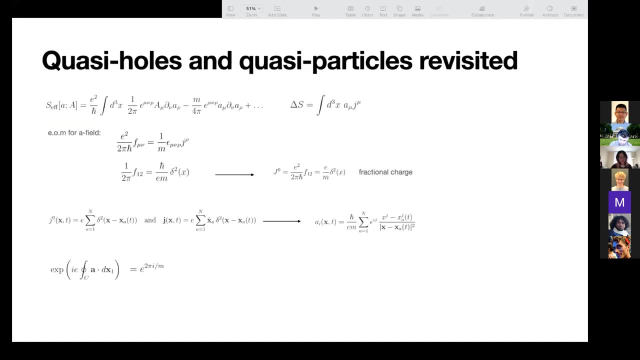 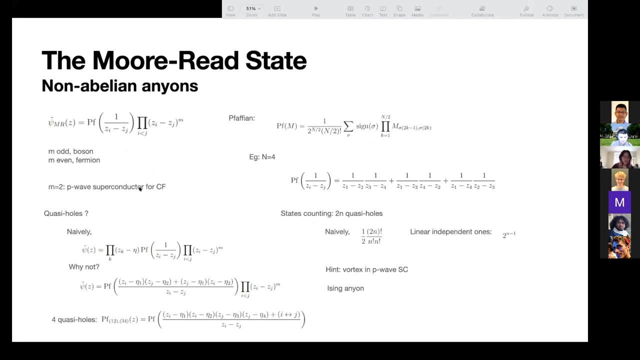 So basically, we just partition four particles in terms of two particles and two particles and exchange indices With some with some sign of the permutation. Sorry, Yeah. So this phaphia, with this phaphia, coefficient times, this guy. 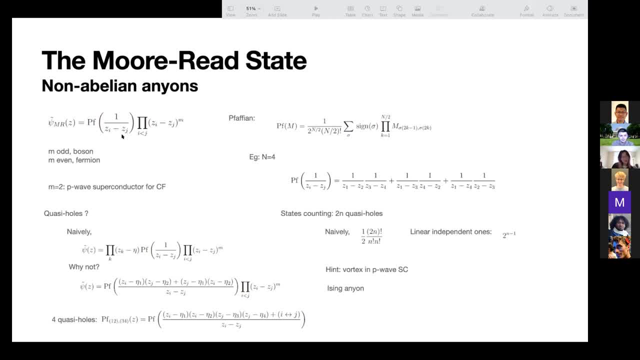 Yeah, it actually doesn't have, actually doesn't have any divergence when ci approaches zj. So this is very good And also because this phaphia is naturally is anti-symmetric. So so this small read state is for bosonic system, where m is odd, and for fermionic system, where m is even. 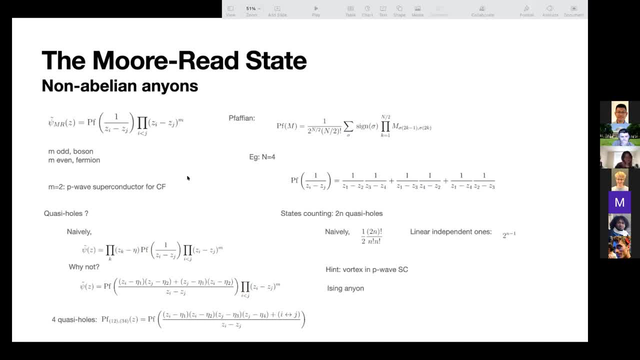 So that's the difference between this guy and the Laughlin wave function. So, interestingly, actually, for m equals two. this describes a P wave superconductor for the composite fermion, So I'm going to show you how to do this. 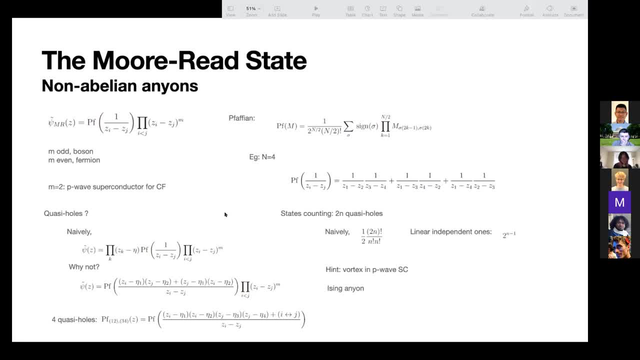 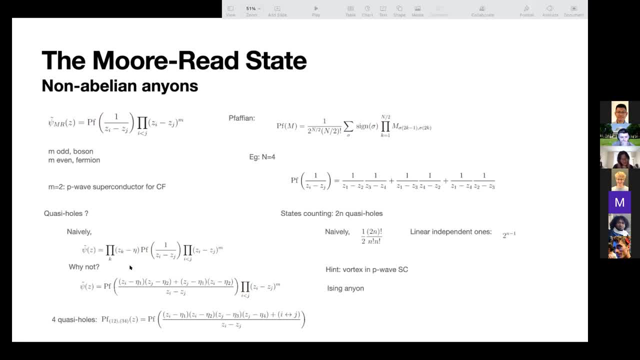 farfian coefficient and uh, and put the, put the, put the, put this coefficient inside the farfian stuff and uh, you can see that when eta one approaching eta two, that this guy, this guy is proportional to this guy. yeah, so that means that means we actually have, uh, we did this, this heart, this uh putative. 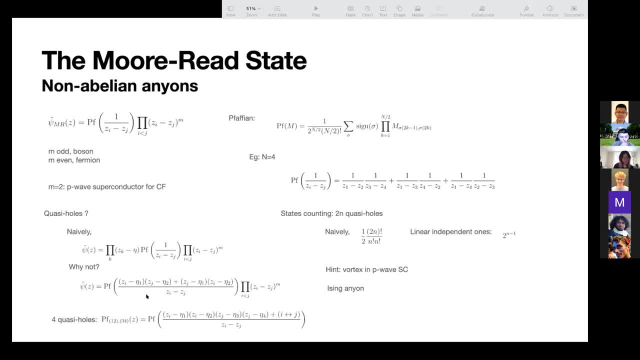 half hole, actually putative quasi-hole, actually splits into two, two quasi-holes. yeah, so that that's very interesting and uh, we can include more quasi-holes in terms, uh, of the coefficients on the numerator of this farfian and uh, so now we want to uh count how many states there are if we have two n quasi-holes. 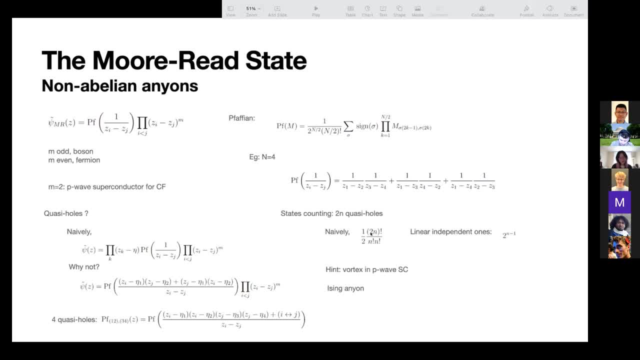 so naively, uh, we divide. we divide two n quasi-holes into, uh, two piles. so naively we have, we will have this much of this many states. but uh, actually those farfian are not linear independent. so the linear independent ones are only two to the a minus one. it's much smaller compared to the naive counting. 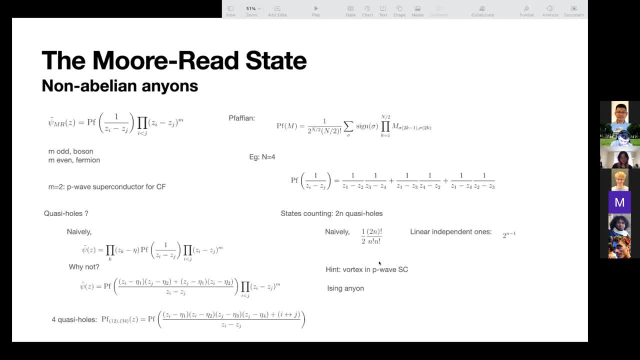 yeah, so why this happens? so, um, as i mentioned, as i mentioned, but as i mentioned before, actually this m equals two- is a p wave superconductor for composite fermion. so this quasi, these quasi-holes, are actually vortex in a p wave superconductor. 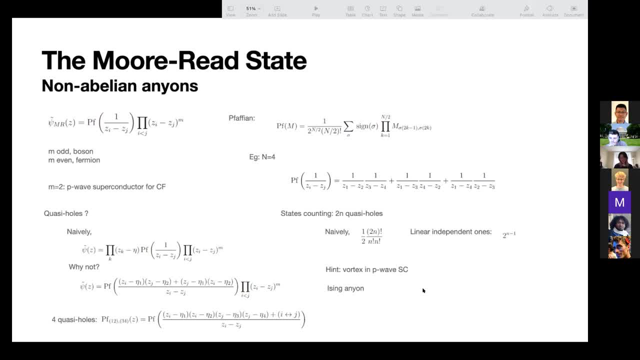 so, uh, if we com, if we uh, if we compute the, uh, the, the bounce, the bounce state of the vortex in p wave superconductor. so, uh, if we, that's T, s, fa, k, Creating a leaf supervisor to build a force action bayonets, a force quarter point to create a died around other Birke and a double bonus. and uh, so we can now we can make this for, uh, saucer. tässä we will find that it's actually a myorana fermion, so that if we have, uh, some myorana fermions and so i mean, we'll need for them to form a. 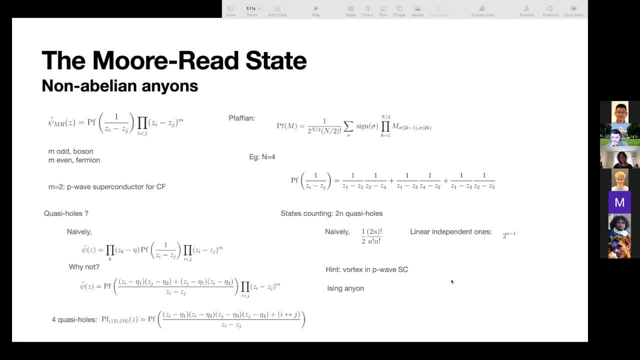 a complex fermions and uh, such that we can have two states, such that we can have two states, hoot it lusciously. uh, look at it, we have two states, such that we can have this complex formula, occupied or not occupied, that spans a two-dimensional Hilbert space. So that's why we get this bizarre number of linear independent states. 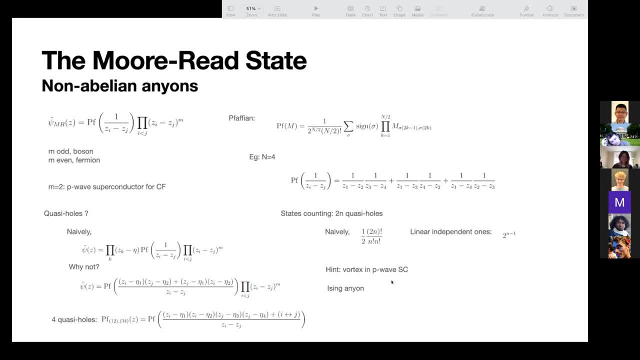 And those, yeah, and if you are familiar with P wave superconductor, this Farfian coefficient is actually a wave function of that superconductor. Yeah, and these vortex, so these quasi-hosts of of the more. restates at M equals two. 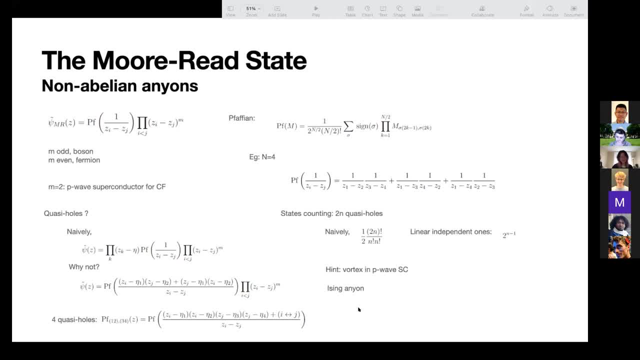 we'll find that I probably will not have time to talk about it. It's actually called Ising annuals. So yeah, so so far this, those wave function approaches looks good, But but when we- but when we are dealing with states like more restates. 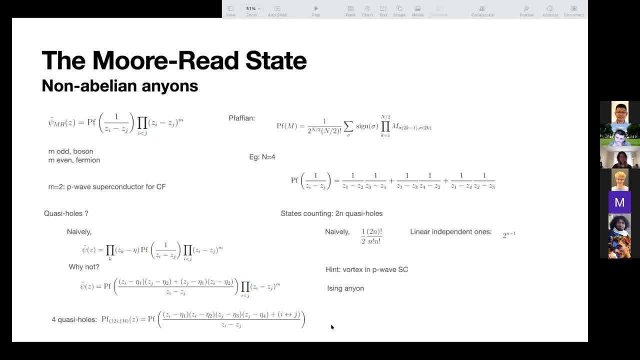 this wave function looks very complicated And it's not. it's not at all obvious how we can obtain the, the statistics of the quasi-hosts, Right, if we want to, if we want to, if we want to compute, say, just the space, just the. 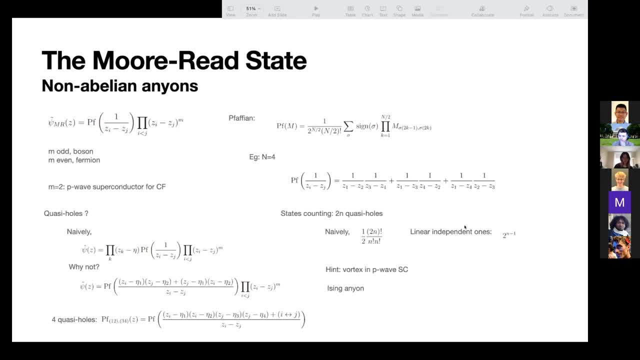 space of the, just the Herbert space, on the quasi-hosts. it will take a lot of effort to try to analyze those Farfian coefficients. So so an alternative way of dealing with fractional quantum. we sort of take a coarse grained approach and think: 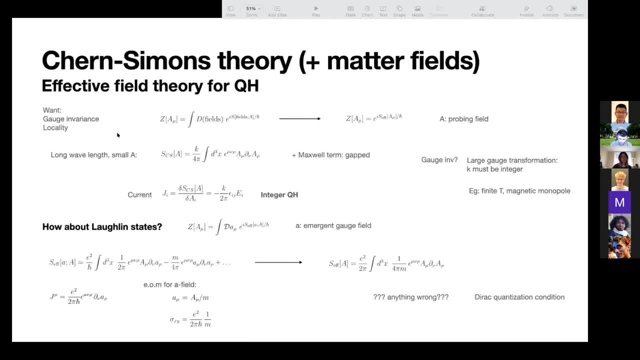 approach and uh, think and think, of what kind of effective field theory that? what? what's the effective field theory for quantum holes? so by effective field theory i just mean, since the quantum hole, the quantum hostess are gapped, we can just integrate out those matter fields and get some effective action with a background gauge field where the gauge 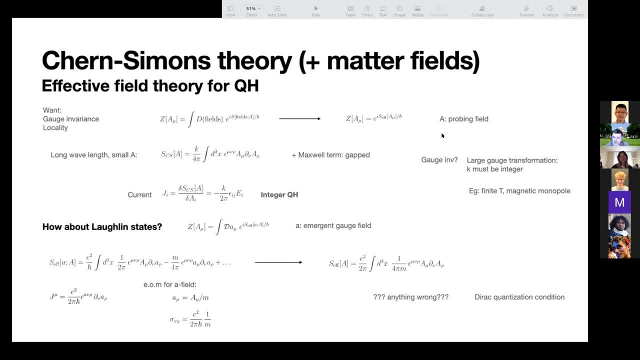 field is a probing field. it's not the. the original um, the original uh gauge, the original magnetic field that caused the quantum whole state is not included in this big a. so from a general concern, from general consideration of a reasonable field theory, we we required the theory to be gauge invariant and so we also wanted to be local, and we're also. 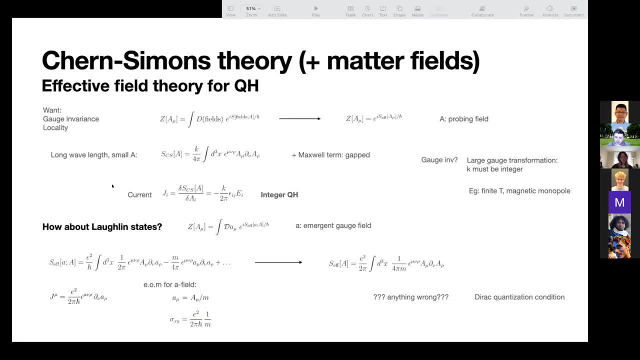 dealing with probing fields. so we want to so want an effective theory at long wavelength and relatively small gauge fields. so there are not many terms we can write down and we can write down them order by order because we're considering this limit. so the leading order term is the 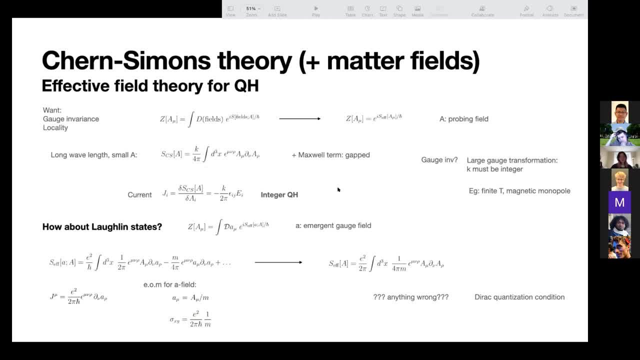 called the transimons term, which looks like this guy, and the next order is the maxwell term. so yeah, so the transimons term plus maxwell term actually gives a gapped photon spectrum. so it's, it's good, because we want to consider gapped theories. 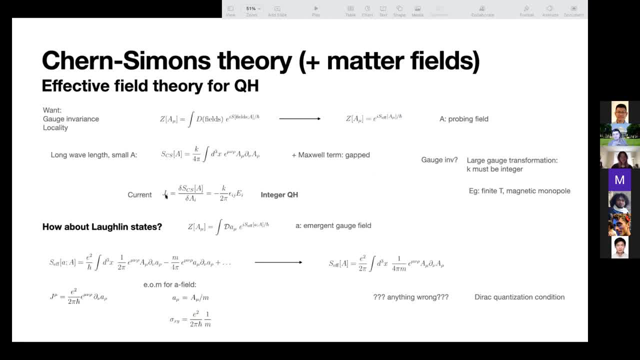 also, if we compute the current of this probing field, it's. it actually gives a a hook, it actually has a whole coefficient, which is also nice. but one puzzle is that this transverse theory seems to be gauge invariant. so I mean, there seems to be no. 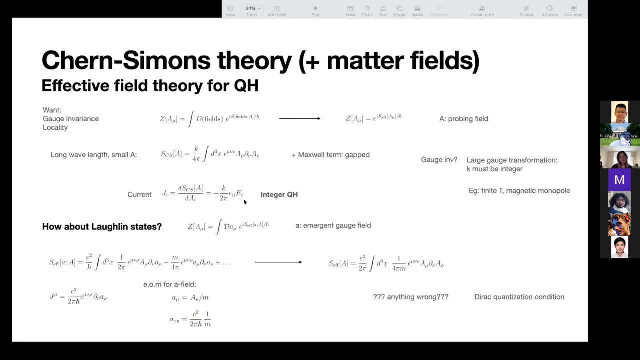 constraint of this whole coefficient. so how does it, how can we relate it to integer quantum law? So actually, if we consider a large gauge transformation, we'll find that this k must be integer. so by large gauge transformation, one gauge transformation we can consider is that: 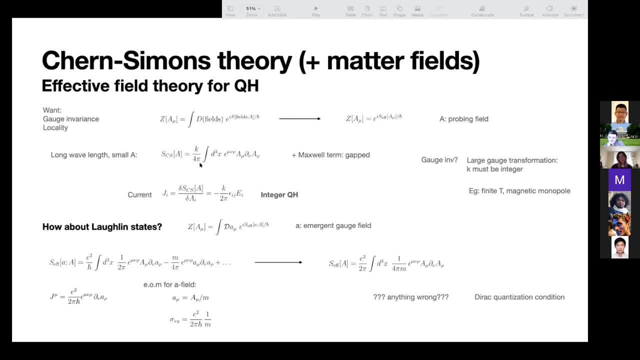 we can put this system. we can turn on the finite temperature, meaning we can do a weak rotation to a finite temperature. Okay, so to consider a finite temperature configuration and make this also make the space compact, consider a sphere and we insert a magnetic monopole to it. 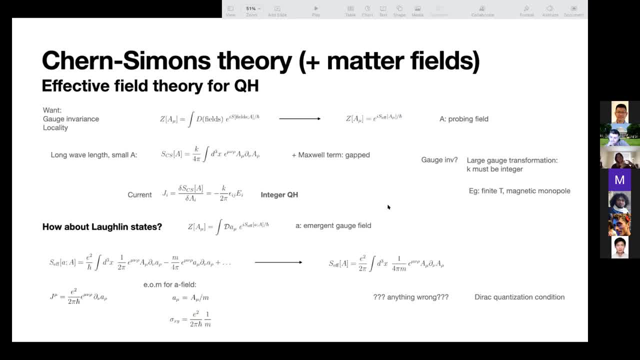 consider the whole path integral. yeah, and we can. for this, for this interaction, we can insert a quantum function. So the gauge invariant actually requires this partition function to be single valued. but this, but this effect to action, can have some face. 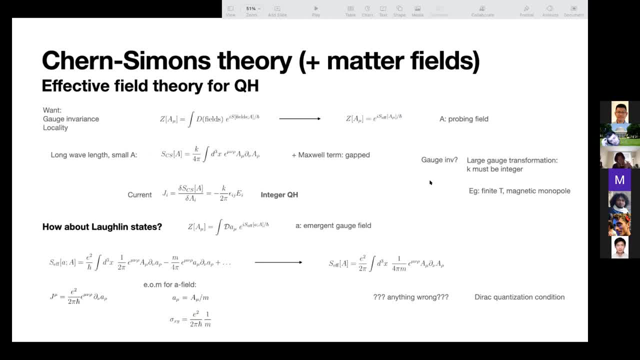 face factor after. after considering that, taking that into account, we'll find that k must be an integer. So, but as we talked before, we can have Loeffling states, which I mean the whole response doesn't need to be integer. 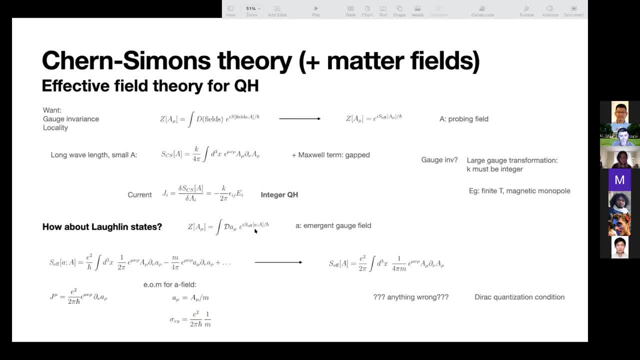 So what happened here? So let's put this aside and just consider another theory: with emergent gauge field coupled to the probing gauge field- And since now we know this term is actually gauge invariant- we can introduce a transcendence term for the emergent gauge field. 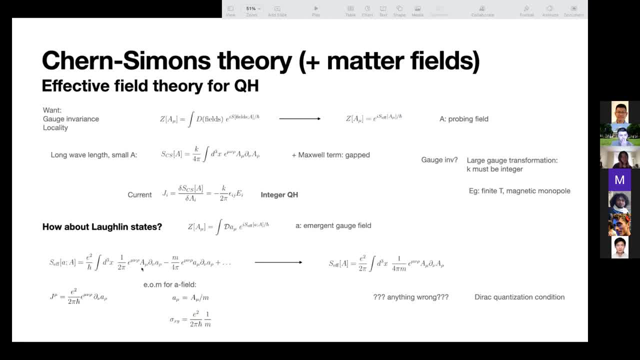 and have a mutual transcendence term between the probing field and the emergent field. So then the current of this probing field is given by this gap And automatically the current is conserved. But if we consider the equation of most of this is auto a field, we will find that 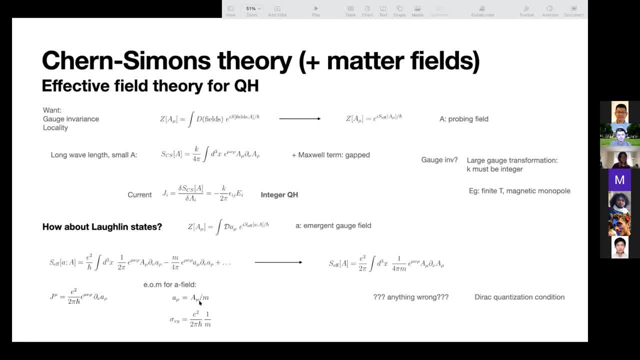 This little a photo is actually one over m to the big a field with some plus some gage stuff. That's what gives, that will give us a whole conductance which is one over m, And if for the more. if we integrate out this, I feel 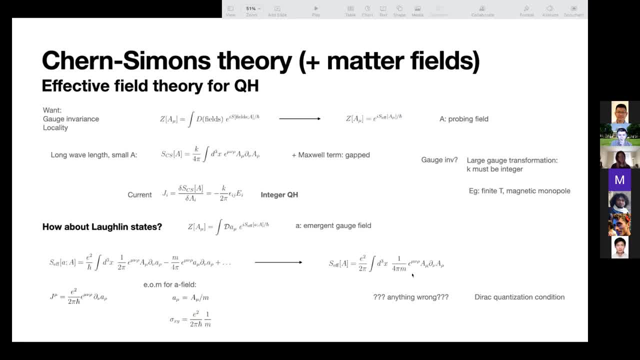 they feel we'll get a one over M coefficient in front of the transcendence term. So that seems. that seems that conflicts with the observation we just had. That mean right. I just told you this: the gauge invariance required this coefficient. 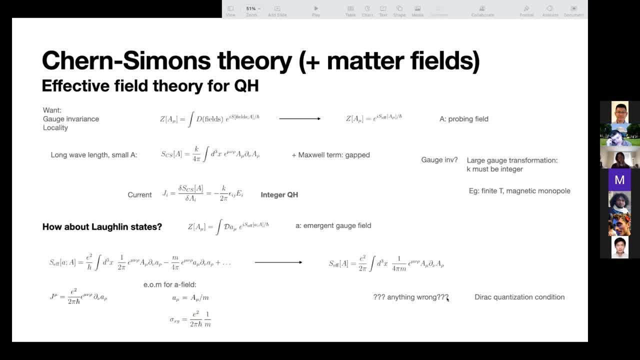 to be an integer. So what's wrong? So actually there's, I mean there's nothing wrong about this guy. The problem is with the Dirac quantization condition. Note that in the large gauge transformation I told you before we insert a magnetic monopole which has a stress. 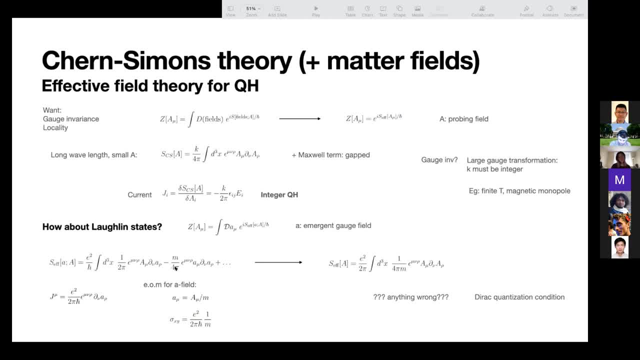 one that's determined by Dirac quantization. But here so. but here for this I actually require the Dirac quantization condition for the little a field, not for the big a field. That's why, that's why we get this one over M coefficient. 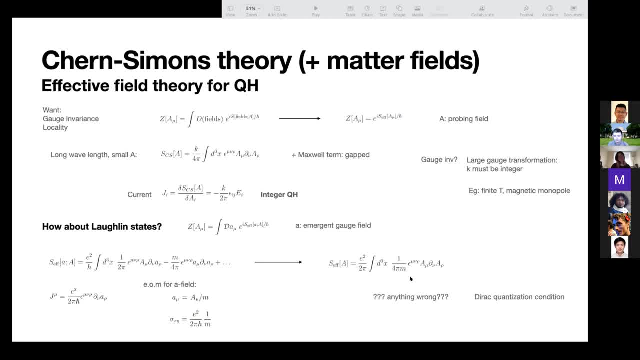 So. so with that, we can see this: if we don't impose any Dirac quantization condition, the coefficient is actually meaningless. We have to specify what we call charge one to. I mean to make those coefficient meaning, for yeah, that's a caveat. 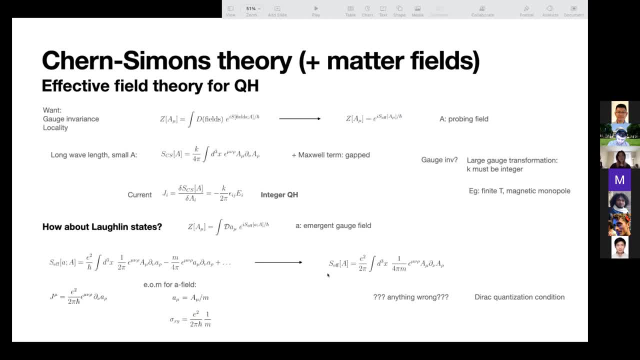 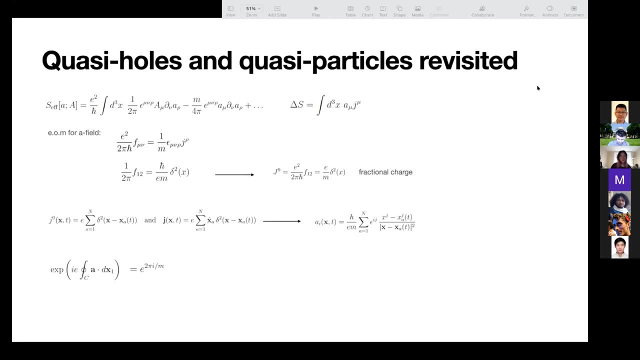 of dealing with transimers theories. Oh, okay, So from the transimers theory we can also, we can also calculate the quasi-hose, quasi-particles. consider quasi-hose and quasi-particles and their statistics. Yeah, that's, I think that's. 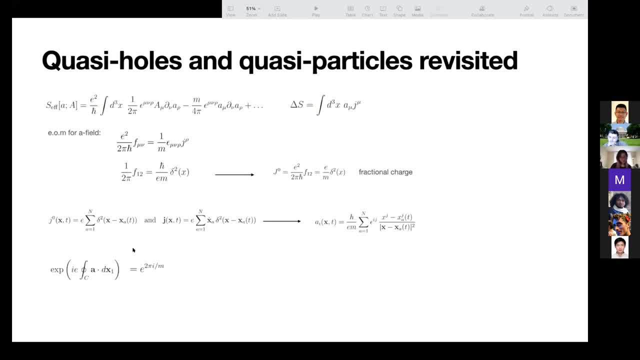 if you, if you take Xiaogang's class- I think this is one of the homework problems- Yeah, basically, basically starting from the effective action we had before and add some charge density to it, So yeah, And if we consider the equation of motion, 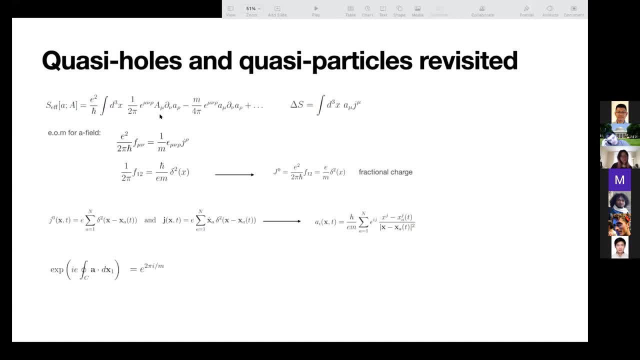 for the little a field and so, and turn off the probing field big A for a moment, we'll see that actually this charge of, yeah, actually the charge, this, this electric charge, is attached with some magnetic flux of little a. 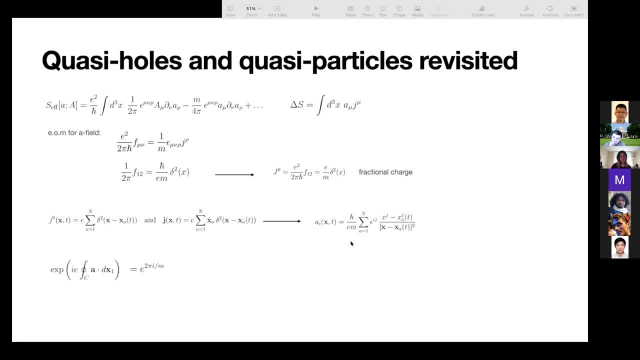 So people often call this flat, flat Flux attachment. And if we plug the plug, the equation of plug, what we get from the equation of motion of little a field back into the definition of the current, we'll find we get a fractional charge. 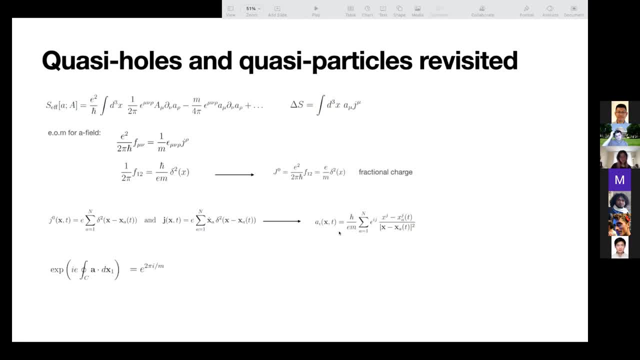 So, yeah, so we can also consider the statistic angle of two, two quasi particles By writing, by solving the- by solving the equation on motion of little a field and and the compute and computing the A- B phase of and. 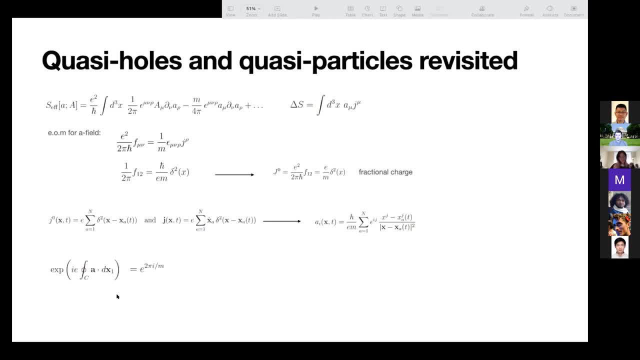 by considering the A- B phase of rotating one quasi hole for the whole around another. in the end, you'll get the same result as we talked, as we talked before. okay, uh, this, uh, this emergent gauge field, considering these emergent gauge fields? uh, looks like uh. 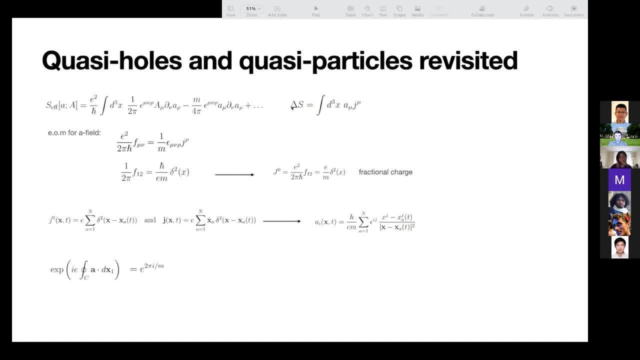 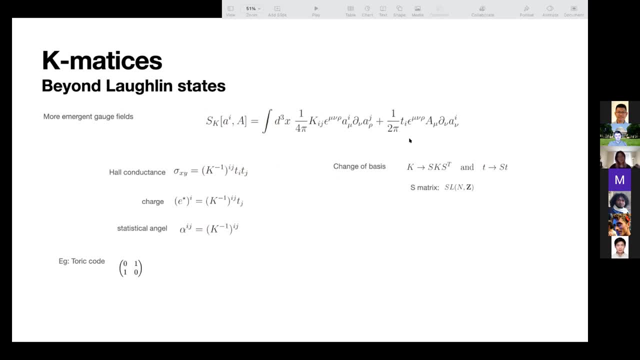 a very promising move. so why not, uh, having more, more of them, so more we can, so we can have more emergent gauge fields and, in general, this effect, the effective action, will be like this guy. so we have a transcendence term between between the emergent gauge fields and 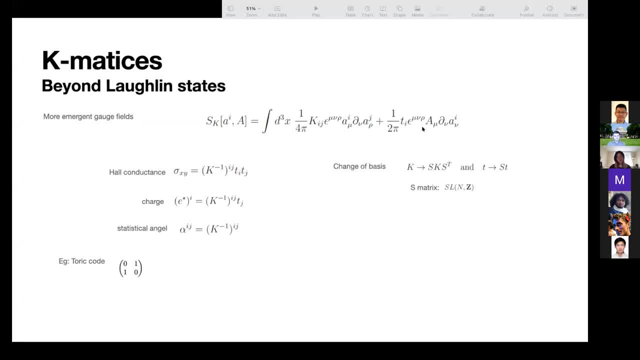 the mutual transcendence term between the emergent gauge fields and the probing field. and the coefficient here is can. it's a matrix, people call this k matrix, so we can also consider the whole conductance, the charge, the statistic angle, uh, the, yeah, uh, you can, you can work out the. 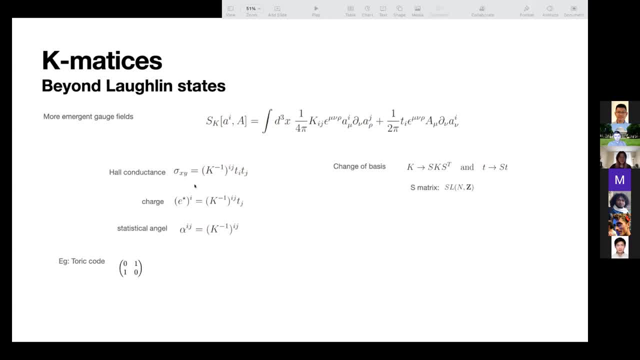 those by yourselves, i think. uh yeah, and they all have this very beautiful uh formulas, sort of the будzis, which is the theondova mezzo- tapa, but but also a kind of an interesting thing to note is that we we also note that a different k matrix and this t. 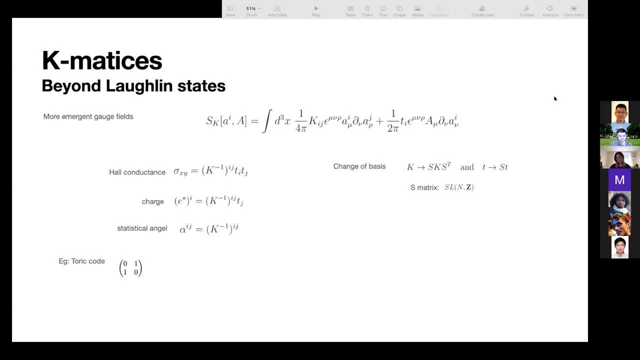 vector doesn't necessarily give, doesn't necessarily give us different states, so there's actually an equivalence relation. that that's uh, yeah, so if we condition. so this equivalence relation is given by this s matrix with, which is an element of the slnc matrices. so, uh, to make contact with uh, what uh, uh, what we talk, what uh people talked before like a. 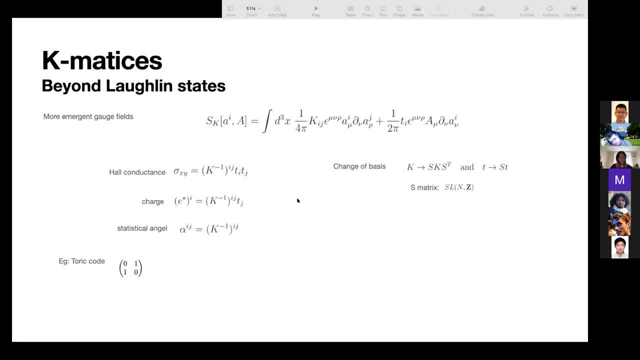 uh torah code, and so so actually this uh k matrix uh can describe uh many others, any many other uh topological orders, for example, such as torah code, although uh, i mean, we can't forget about this coupling to the probing field for now- but uh, for this k matrix, the, the k matrix for torah code is: 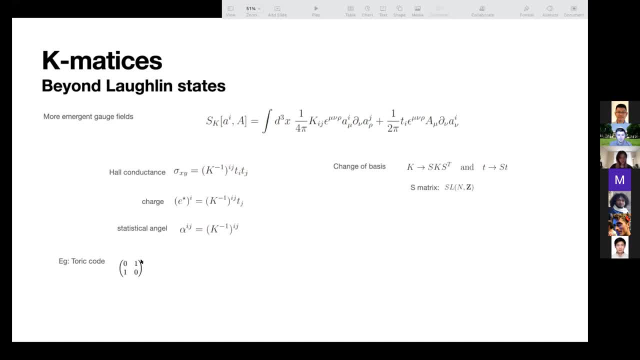 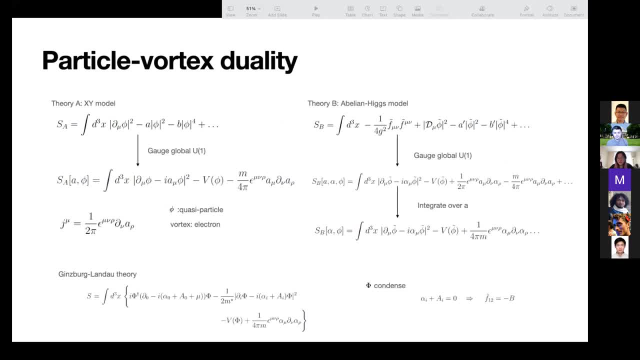 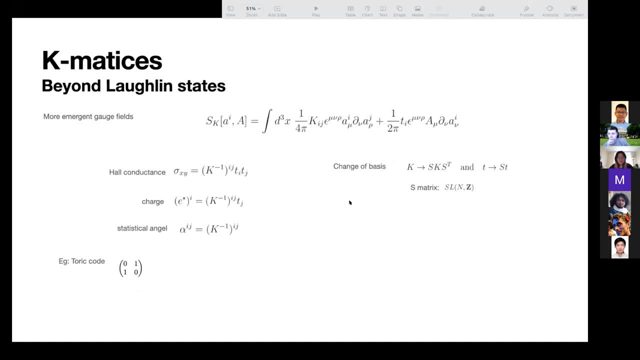 uh, okay, uh, so, so we talk. so so i tell you that this uh effective hamiltonian can describe uh quantum post-states. but uh, we can also put, we can also put the uh matter field back and make the so so this effective action is integrate over the. 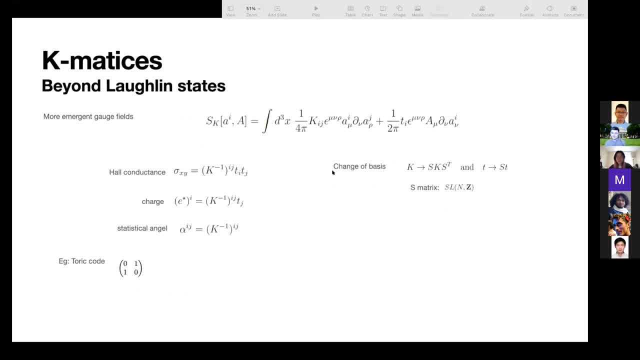 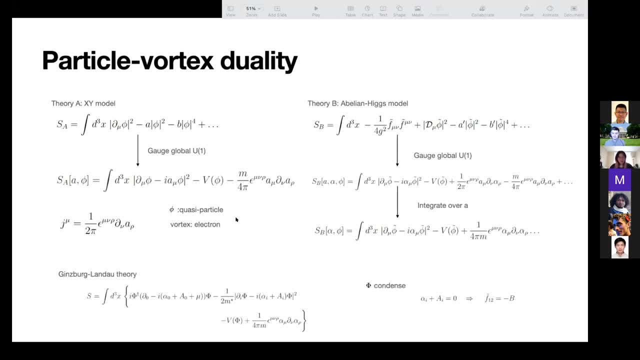 the matter field, so we can also put the matter field back to see what, what happens, yeah and uh, actually this, uh, So, yeah, so I actually want to talk about the particle-vortex duality. In the particle-vortex duality, on one side we have the S-Y model, on the other hand, 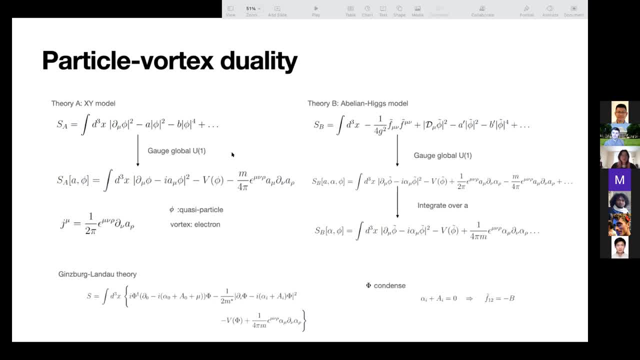 on the other side we have the Abelian-Higgs model. So we have a global U-1 symmetry on both sides. and if we gauge that global U-1 symmetry with a dynamical gauge field, little a- and now we know that we can have transimers term. 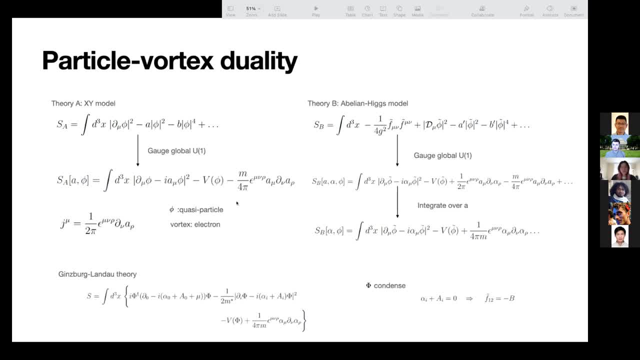 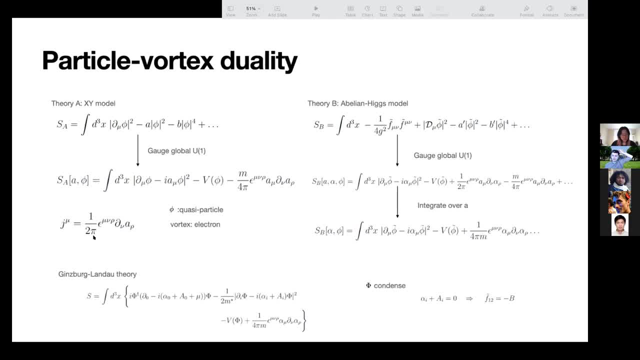 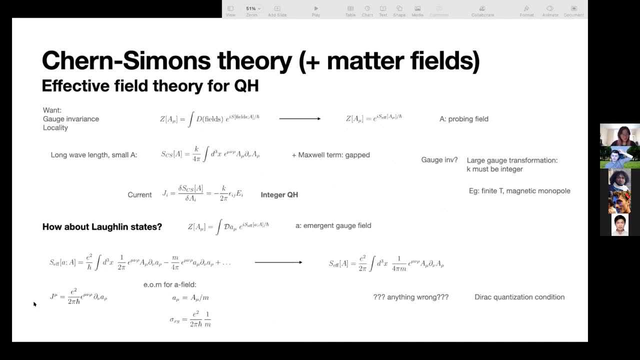 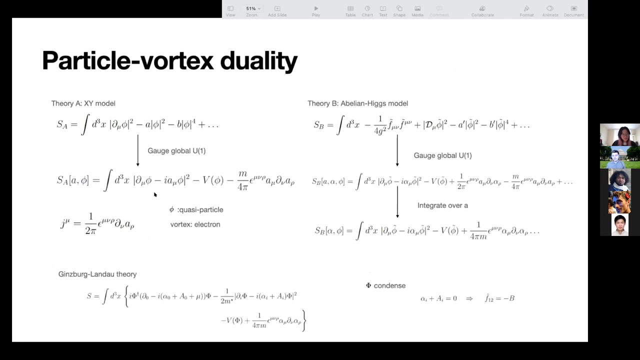 So if we consider the current is actually given by this guy, it looks a little bit like. It looks pretty much like the current we have. Okay, the current we have here. Okay, the current we have here, Yeah. so that means in this description of this S-Y model, if we couple it to: 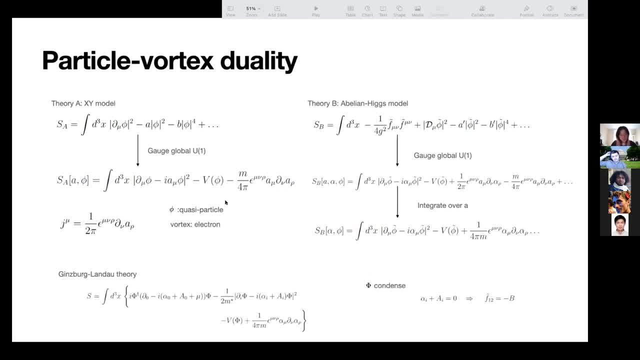 We can also couple it to a probing field which I didn't write down. So yeah, so then this vortex is actually an electron and thus the phi quantize actually gives the quasi-particle. But we can also see that in the dual description. 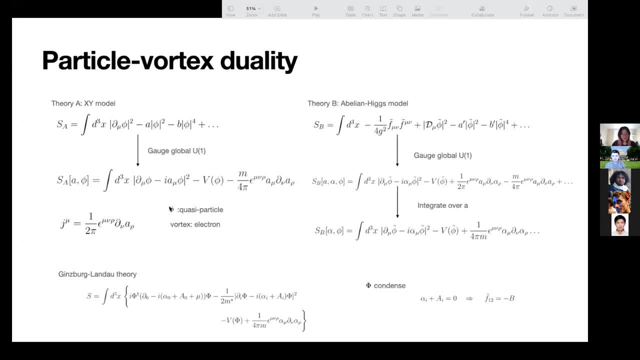 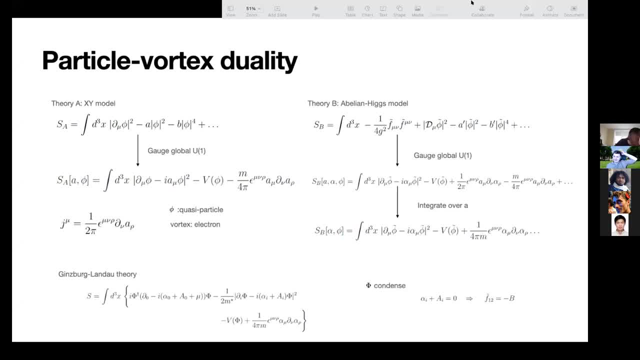 Let's see, I think we're a little over time. Let's see, I think we're a little over time. Sorry, No, that's okay. What, What, What, But Yeah, so just like, maybe in five minutes. 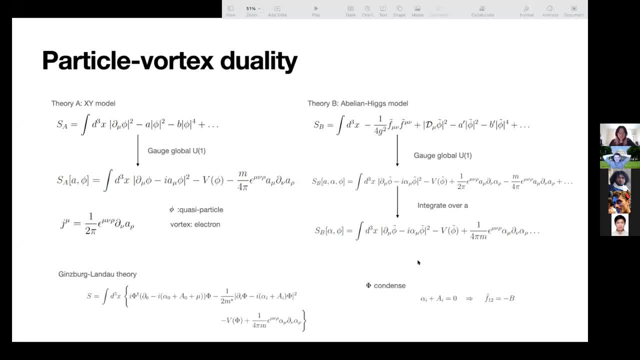 I don't know. Oh, yeah sure, Oh, yeah sure, Oh okay, Yeah sure, Yeah, sure, So Okay, diagram of both sides and uh, and work out, uh, you know, so, if uh say yeah and and match, match the face diagram of both of the two sides also, uh, 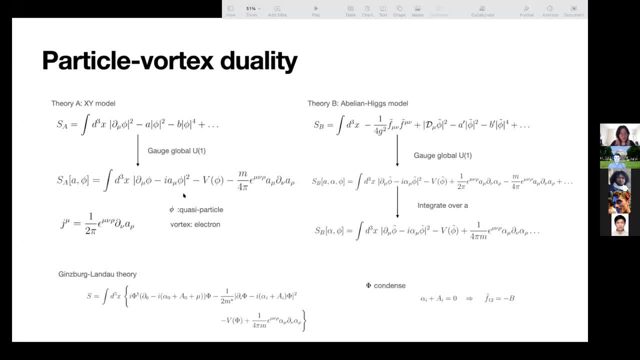 i mean in this uh, in this language of particle vortex duality. this five field is actually has anti-particle uh and uh people also, and people in order, if, if, if you want to get a landau, ginsburg, landau theory, uh, plus the translamism, you need to consider uh actions. 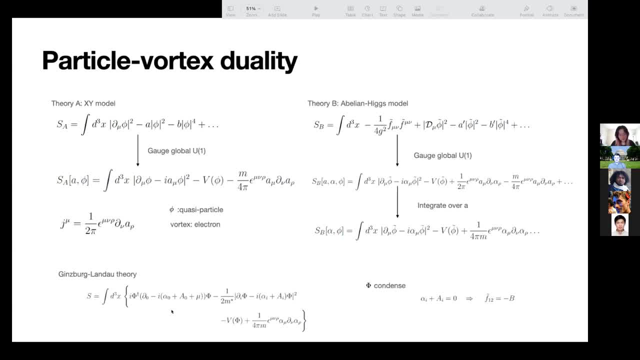 like this guy. so we're no notice that we replaced that. here this five is relativistic and here this little five is actually not relativistic and we put a chemical potential to it. yeah, so i mean, at near critical point of this, uh, superfluid insulator transition. 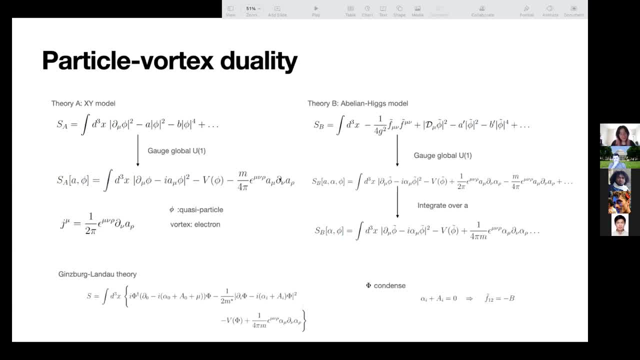 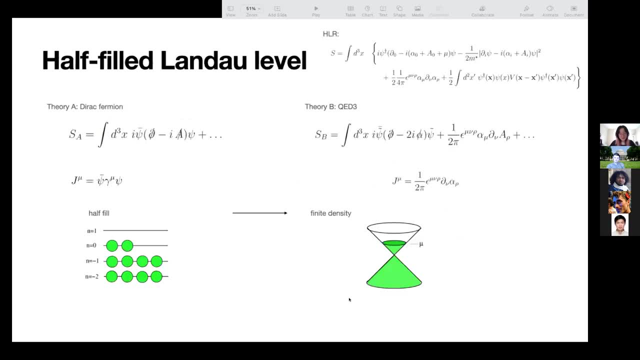 these, these two theories should be, should have same, should be the same, yeah and uh. and we can also consider half field landau level and a couple of other theories and do the duality. but yeah, but it's uh, uh, it will be a very long story. 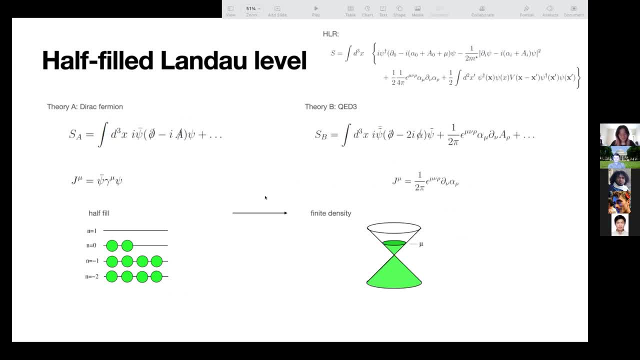 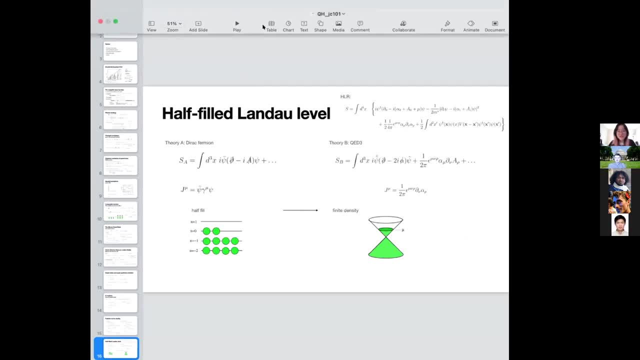 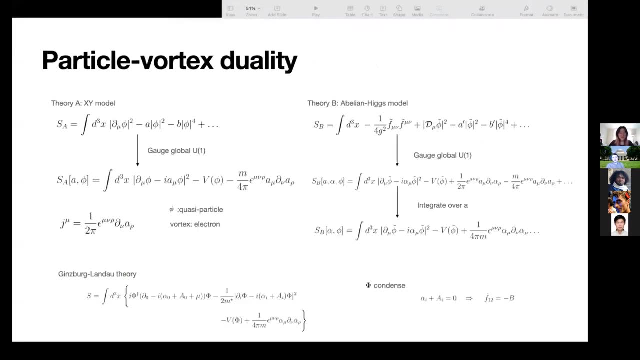 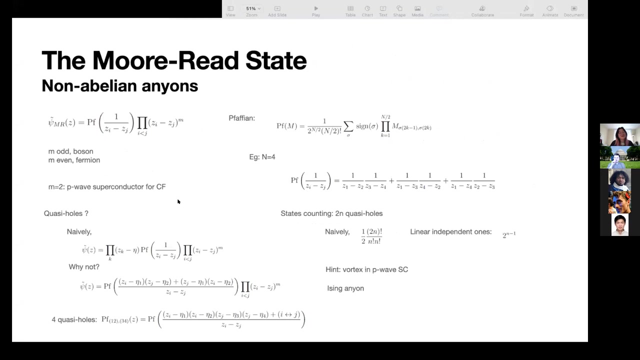 for this for this half field, landau level. so i'll, i'll stop here. thank you, yeah, i. so i had one question: um, uh, the when. when you wrote down the moore reed state, you said, for m equals two, it's a p wave. uh, superconductor, yeah, yeah, and so i was wondering if, if there's any physical way to. 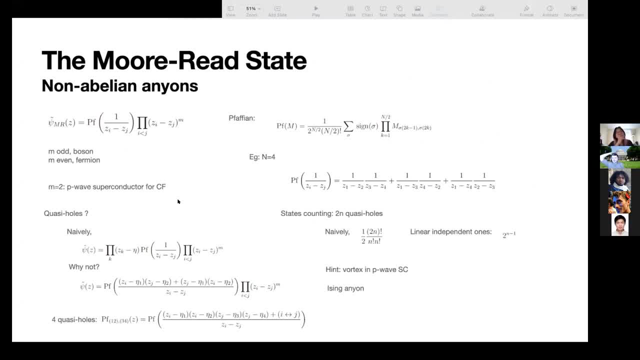 understand this like: is there some sort of instability to, to pairing, or is it just like we're writing down this state and it is the description of a p wave superconductor? yeah, so the stability question really depends on the hamiltonian right, right, so Yeah, but here I just propose some kind of 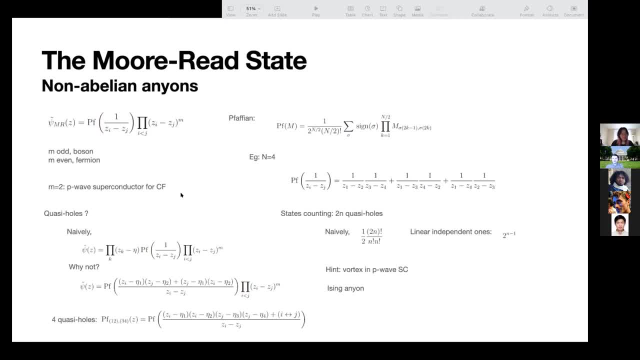 I just propose a wave function for this state. I don't have any. yeah, it's not a statement of the instability. Got it Okay, thank you. Yeah, I have a question. So you were talking about how the Chern-Simons term 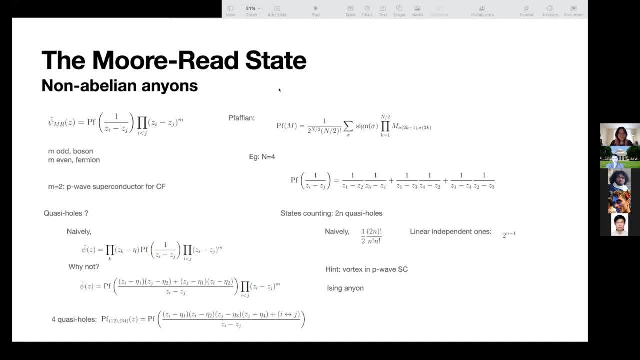 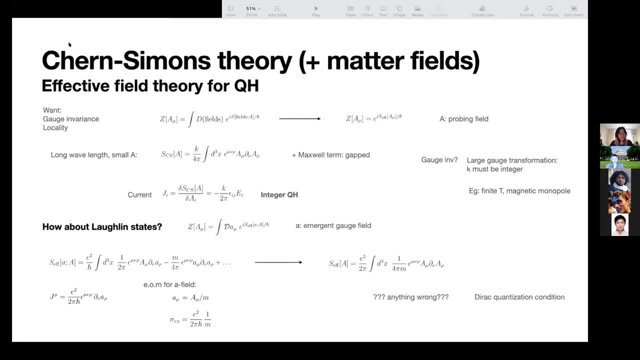 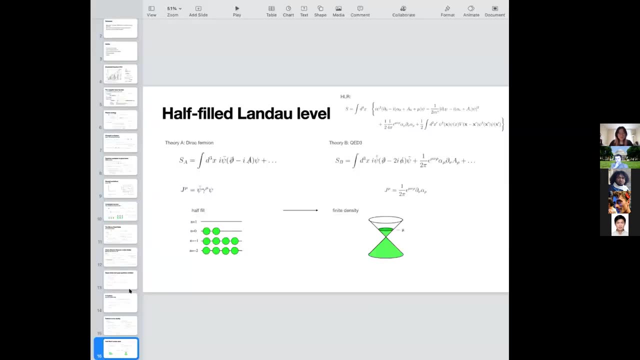 plus a Maxwell term leads to a gap for a gauge field, right? Yeah, Yeah, you said this is like what we want, sort of, but I don't know, it's kind of surprising, right? You like you couple a gauge field to a bunch of gap stuff. 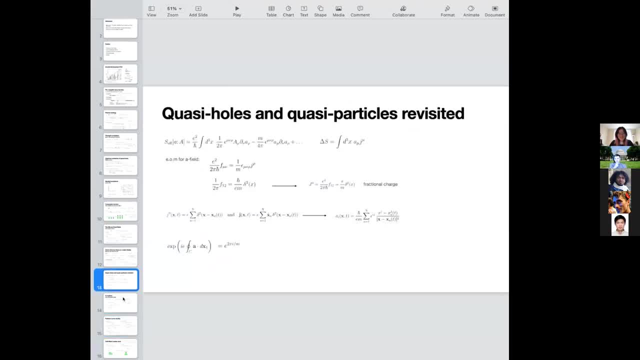 and then somehow that gap stuff manages to produce a gap in the gauge field itself, right? So why did we expect the response theory to have a gap? Oh, I mean, I said that, based on that, we want to get an effective field theory. 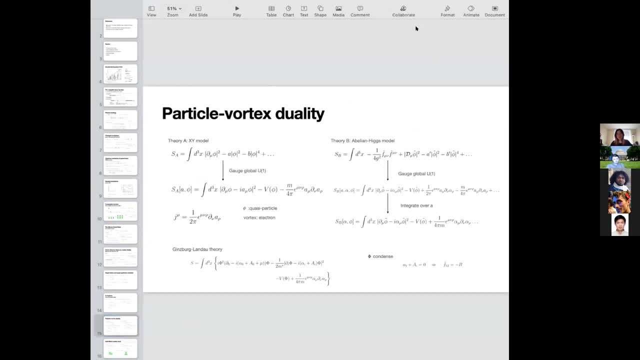 for quantum-core states, right. So we want a gap, So we want it to be gapped. Well, let me think so the matter is gapped, right, But so I don't know technically. So the and but the matter, for maybe do you know, Do they do? they are the matter of the field. Do they seed gapped? Do they feed? or do they, if anything, so they could feed? or like the daguerreConf, that like heavy milk to feed, or in the liquid whenever the��. 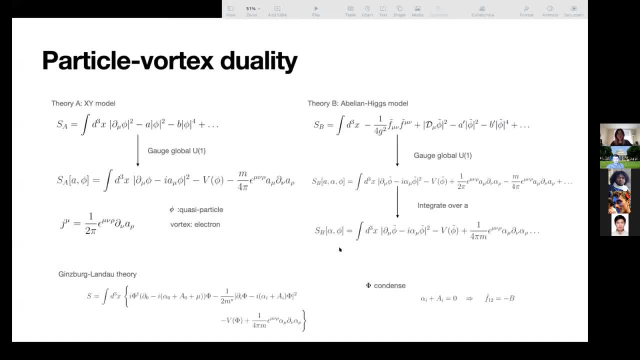 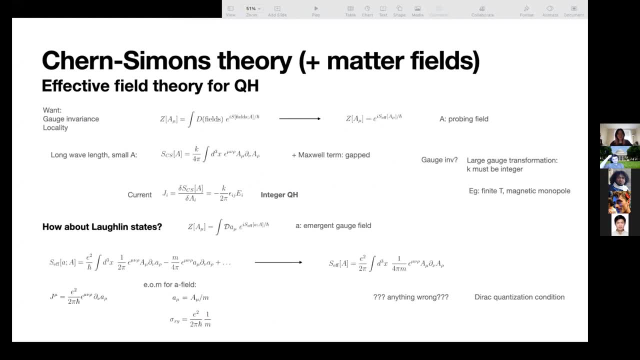 But so am I correct in imagining that capital A should be thought of as like the electromagnetic field minus the magnetic field that's causing the quantum Hall effect? Or is capital A something else? Yeah, right, right, OK. But if I were to just couple A to a massive field, then 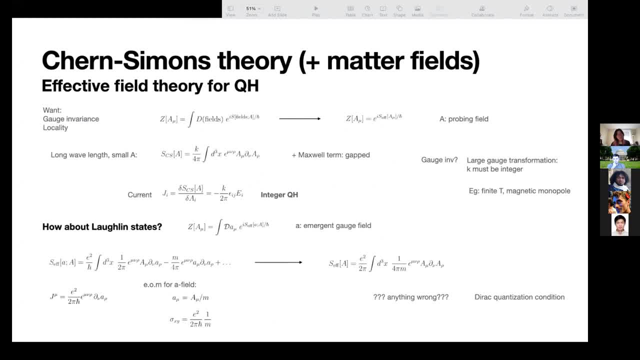 coupling A to a massive thing, then A would definitely not be gapped. I would just ignore the coupling to the massive thing. And so here, if I don't add any A, I have a bunch of gapped matter. But then the claim is that I can couple A to this gapped matter. 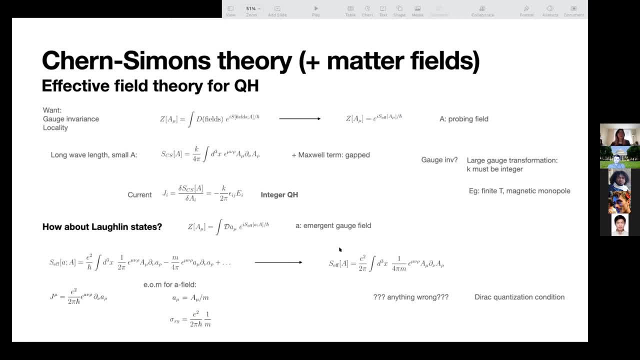 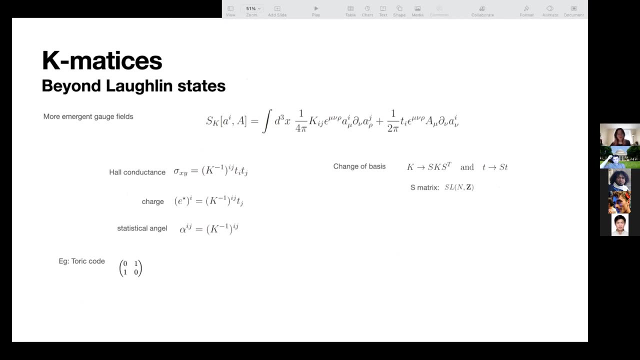 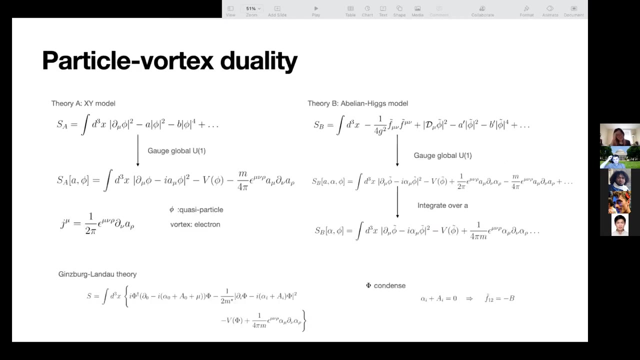 and it'll produce this quantum Hall and then lead to a gap in the A, which is kind of interesting, right? Yeah, I mean, one way to think of it is in terms of this, in terms of the HLR theory, right? 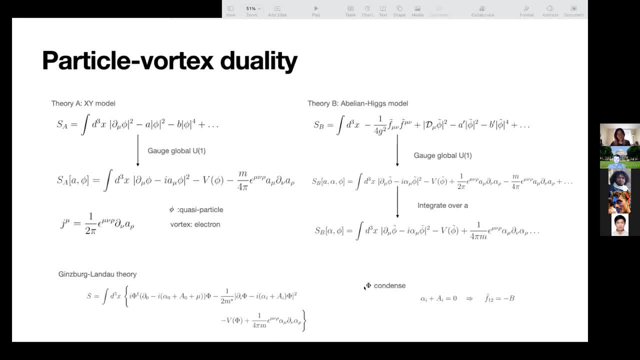 It's like: yeah, it's similar to something. It's something like this: Yeah, you have to. you want to be coupling A to like a Higgs field or something, right? But yeah, I guess that's pretty obvious that this is what's going on in quantum Hall, right? 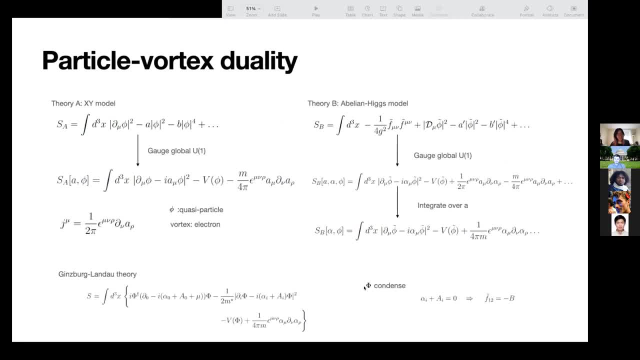 OK, maybe you're saying that using particle vortex duality is the best way to understand it. Yeah, I think that's one good stuff about particle vortex duality, OK, And then so the other question: OK, OK. So the other question is then: I mean, 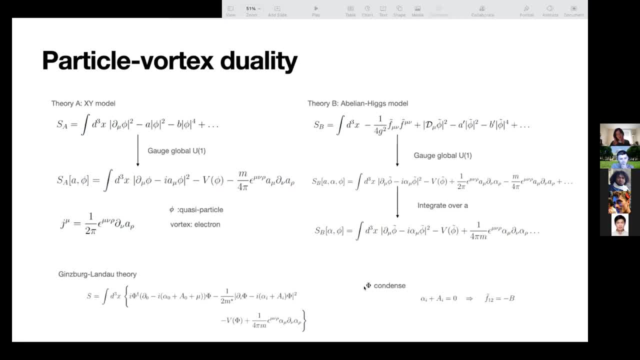 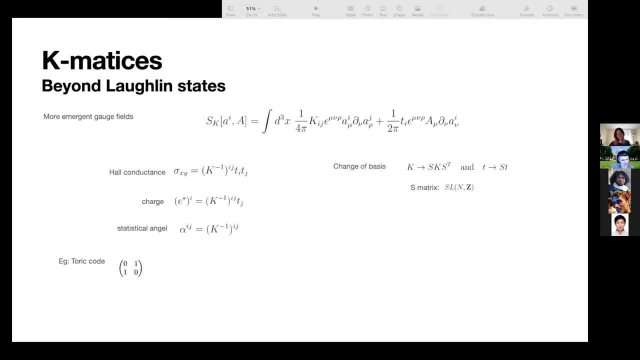 you were talking about the direct quantization condition being important. Yeah, yeah, yeah. So, but if A is supposed to capital, A is supposed to be like the physical electromagnetic field minus the magnetic field part, then I mean in like a real 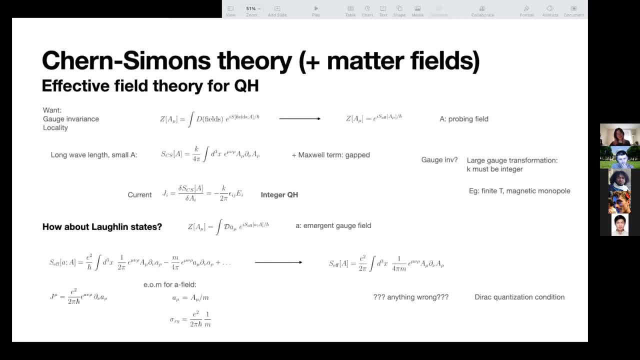 in a. this is too pedantic, but like in a real sample capital A should still have its quantization condition fixed As in a normal charge 1 field, right, Yeah, Like if it's the physical electromagnetic field, right? 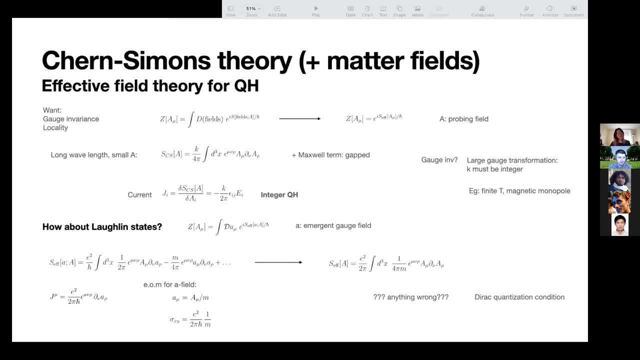 So are we just saying that it's impossible to consider like a scenario where you only have one source, you only have like a 1-mth flux or something, Because there are no field configurations where you can create a 1-mth flux? 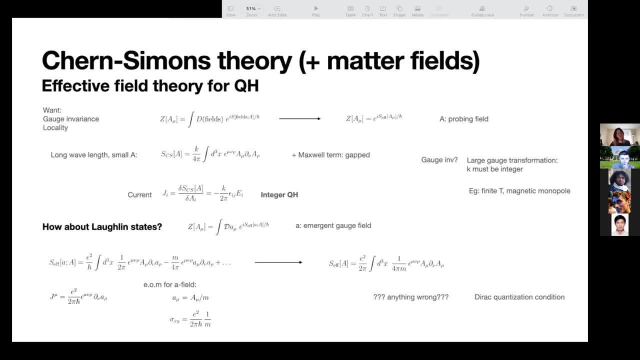 There's no 1-mth charge in reality, So that's why it's OK You're saying so. And also, this equation of motion is equating the field strengths, not the gauge fields themselves. Yeah, yeah, yeah. 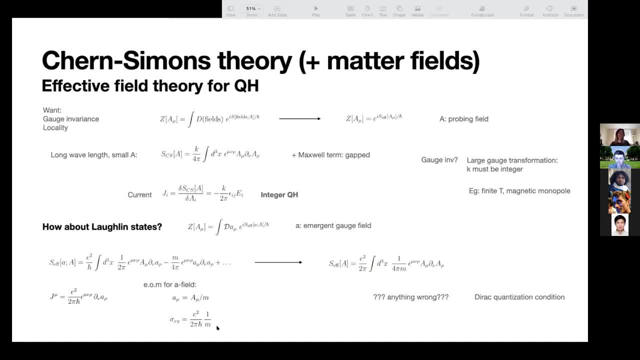 So there should be plus something. Yeah, I didn't write it down. Yeah, yeah, This is an equation of field strengths, Right? So yeah, So back to the question. But the field strength doesn't care about this holonomy part, right? 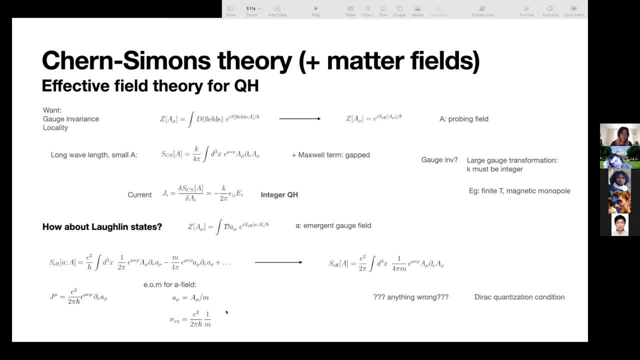 If I just say the two field strengths have to be equal, then why do I say A Right Yeah, But at the end of the day you get something that's so the field strength doesn't care about this derogation, But at the end of the day, we want the effective action to. 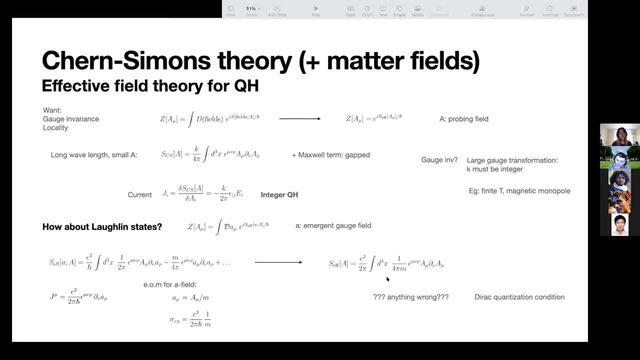 we want a gauge invariant theory, right? So I mean, it's still a question. It seems that by putting a non-integer in front of the transcendence term, the theory might not be gauge invariant. Well, yeah, And I would say that that's true, because the equation of motion 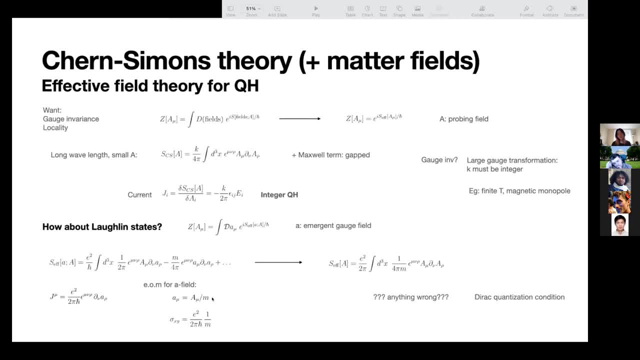 you used was not the real equation of motion. What do you mean If you're using the equation? I agree, you can use the equation of motion to set the third, But then you're saying that the field strengths equal to each other, right? 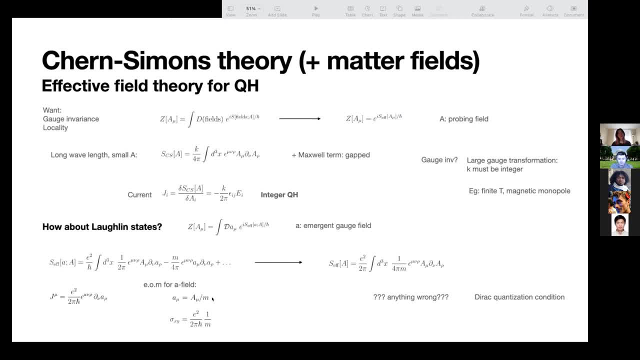 Yeah, But how do you know that it seems like you get- I mean, it seems naively that you get- something that doesn't make sense if you also set the gauge fields to be related by its factor of 1 over m right? 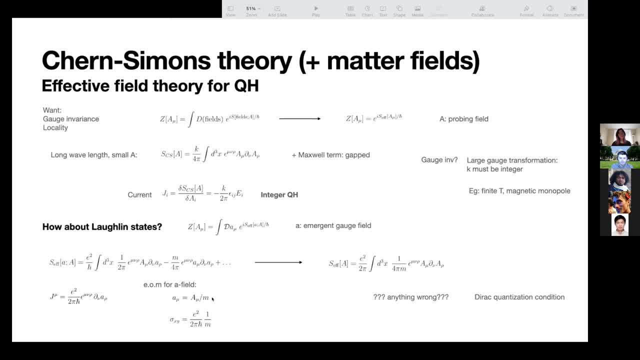 Yeah, yeah, Yeah, that's true. So I would have thought that we ran into a problem because we used- we pretended- like the equation of motion was for the gauge fields instead of the field strengths, right, But then you're saying that there's actually no problem. 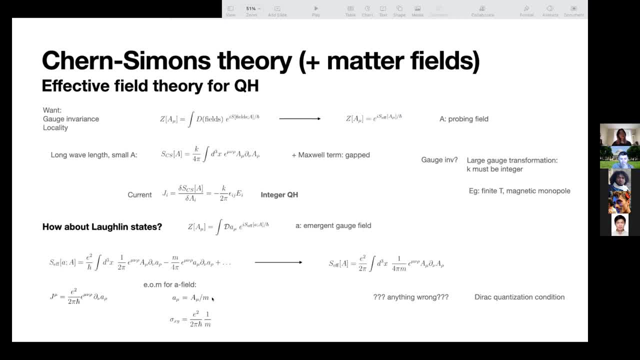 And that using setting the field strengths like this to be related in this way actually makes sense, right? Yeah, it actually makes sense. I mean, locally it doesn't care, The field strength doesn't care about this monopole stuff. 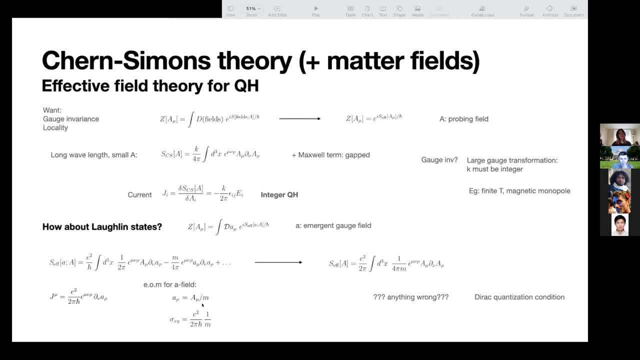 I mean this is a legitimate equation, But the, so the, but the direction, the direct quantization for capital A should still, should be the regular thing. right, The direct quantization for capital A. Right, So this s effective with the 1 over m. 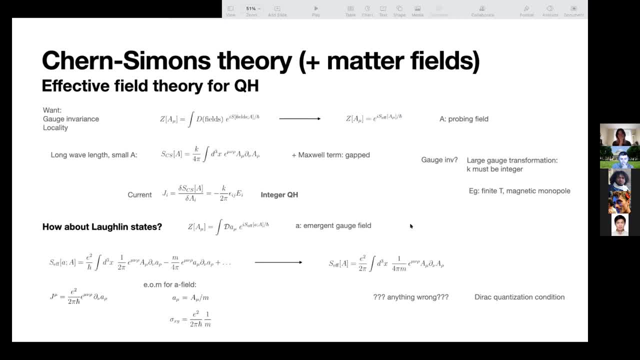 would make sense if I could only consider magnetic fluxes of strength m for A right Capital A. Yeah, right Yeah, But capital A is the physical electromagnetic field, So I can definitely, I can definitely consider a 2 pi flux for capital A right. 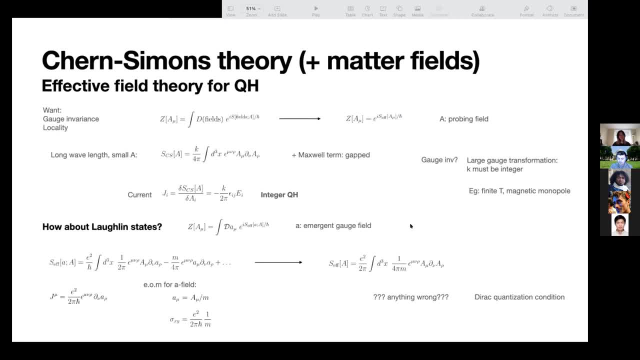 Yeah, you can definitely consider a 2 pi flux for capital A, But yeah, But then don't I doesn't. isn't there something, indeed something, wrong with that? Uh, let's see, OK, Uh, But considering uh, yeah, I, I know, uh, so, so you're saying that there. so the direct quantization condition by capital A should uh always given by I mean by the original one, because because, uh, um, the fundamental electric charge is always E, it's not E over m. 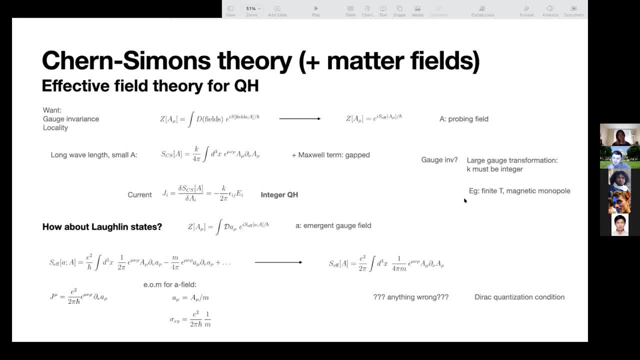 Right, Right, Right. But uh, here we are con, yeah, we're actually we, we tried, we're actually considering a, a quasi, a, quasi particle in this system. Uh, we're, by quasi particle I mean we, we have, we can have m uh, if, if we uh, if we just if we consider inject an elec electron to the system, it will just split to m, quasi m. 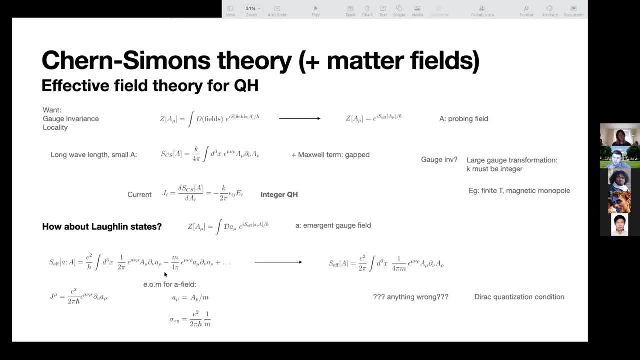 Right, Right, Right, M quasi-particles and then they can move arbitrary far from each other. Yeah, so can I just say that this is equivalent to just pretending like I can consider configurations where there's only one quasi-particle. 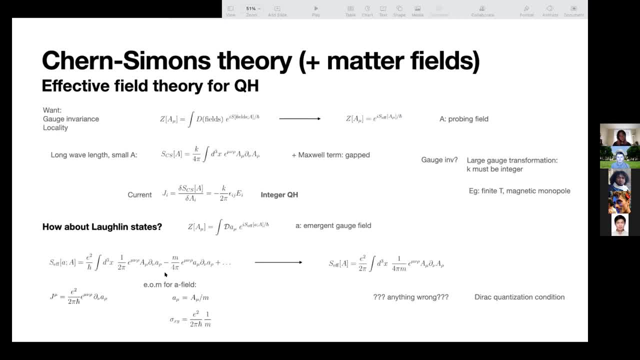 Yeah, yeah, Even though that's not gauged invariant under the little a, Mm, that's gauged invariant under little a. That's not. that will cause this term to be not gauged invariant. Hmm, Okay, I'll just ponder this. 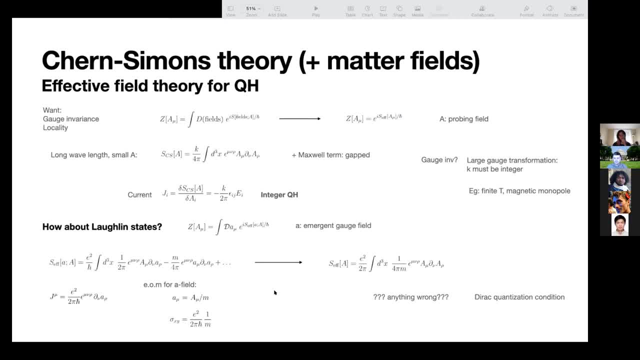 Thanks Cool. Any last questions? Oh yeah, and so you kind of said this. but the Fafn? right? so the only thing I know about the Fafn is that it's a partition function. The partition function for Majorana. 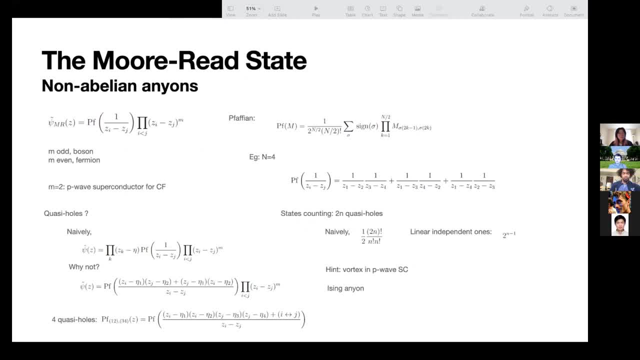 Is a Fafn right. So what is the kind of? I guess you're telling me the answer here on the slide, but like, if I had a partition function where the like action for the Majorana Fermions had this like zi minus zj thing, then that, and then I integrated out the Majorana Fermions, I'd produce this Fafn. 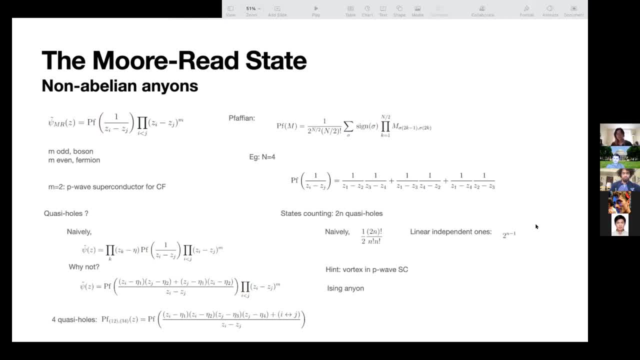 So is that? is there some physical understanding for this? That's coming from this Fafn, that's coming from the Majorana Fermions in this way, By physical, I think, by physical understanding maybe, maybe you can think of it in terms of composite Fermion. 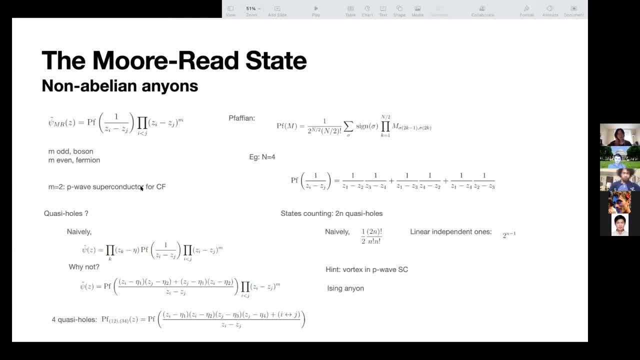 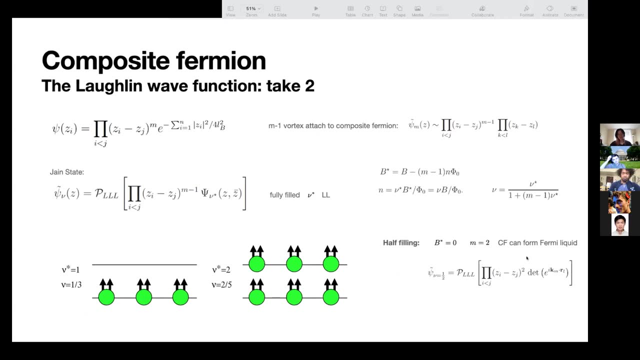 Yeah, I mean in terms of composite Fermion. this, this is a P wave Superconductor for this composite Fermion And, and I think you can get- you can get this by starting from the composite Fermion, Fermi liquid. 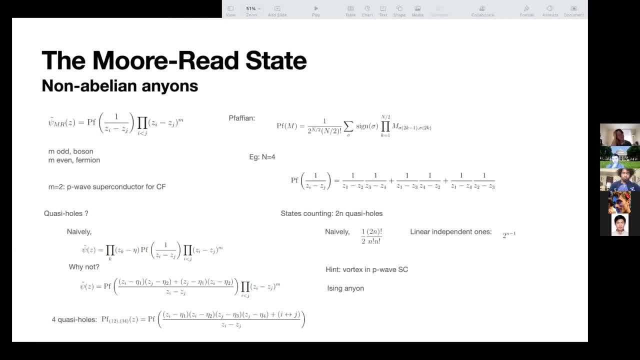 Yeah, Okay, yeah So. so it's like it's just like Slater: anti-symmetrizing, But for real Fermions. Yeah, Okay, thank you, Sure, Thank you. It was a great talk. Thank you for listening. 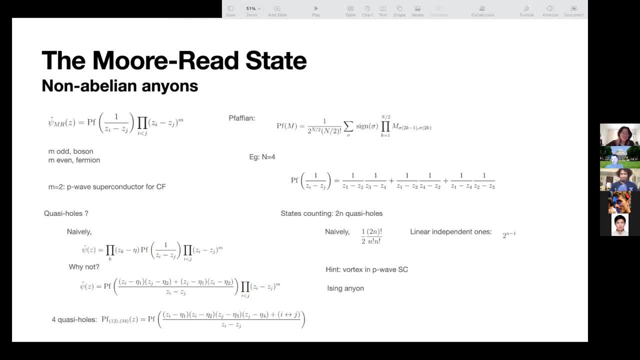 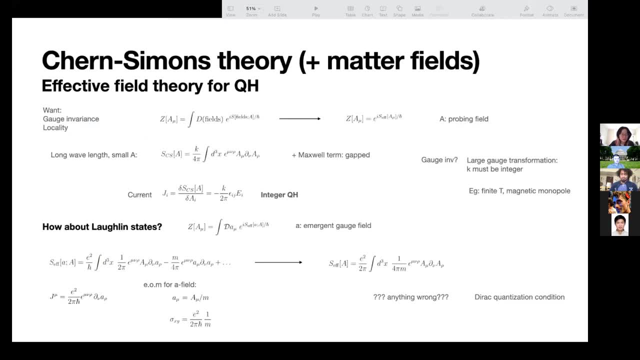 Yeah, thank you. Yeah, All right, uh, i hope everyone has a great thanksgiving break and i will see you um in two weeks when we hear from uh g1 about dmrg. yay, cool, thank you dan. thanks dan, thank you again.